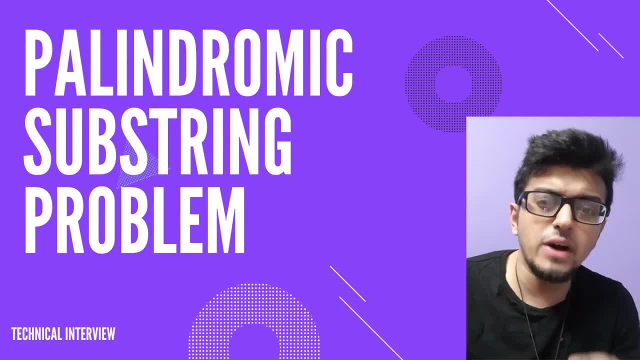 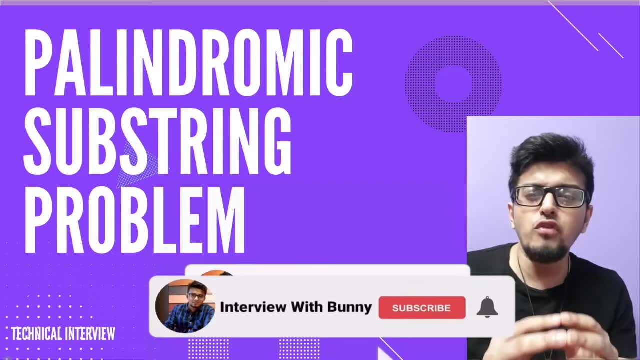 Do you know? according to google, problems on palindrome are the most commonly asked question during the technical interview. Hi, my name is Anindya and welcome back to my channel and over here today. with the help of a single solution, we will be solving five problems for our technical 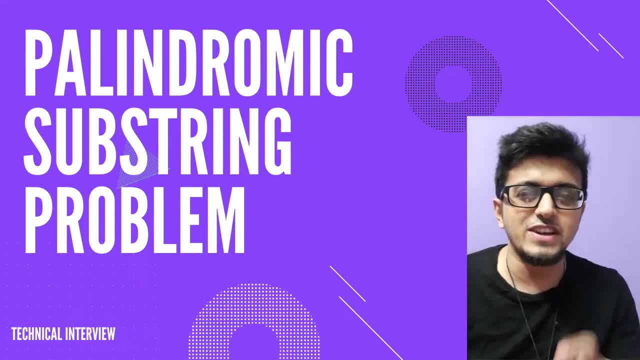 interview. So it's more like five problem, one solution. So, without wasting much time, let's start with today's video. but before that, if you like this video, please do like and share this video. and if you are new to my channel, do not forget to subscribe to my channel and hit the. 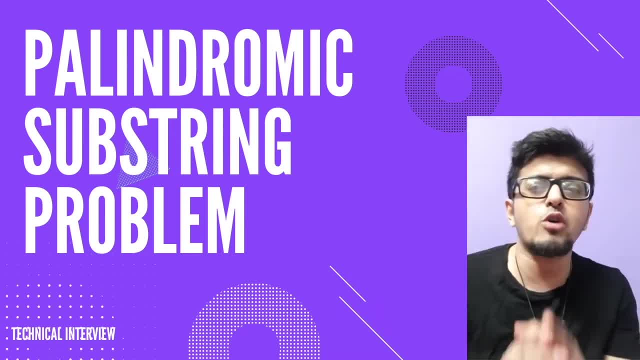 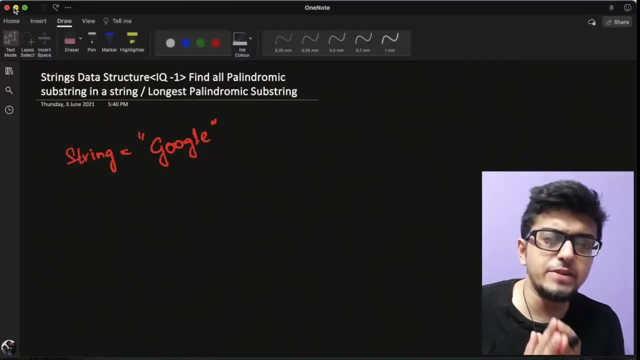 bell icon so that you never miss an update from my side and you're always ready for your next interview. so today we will be solving two most important problem. The first one is we need to find out all the palindromic substring in a string. and 2, we need to find out the longest palindromic. 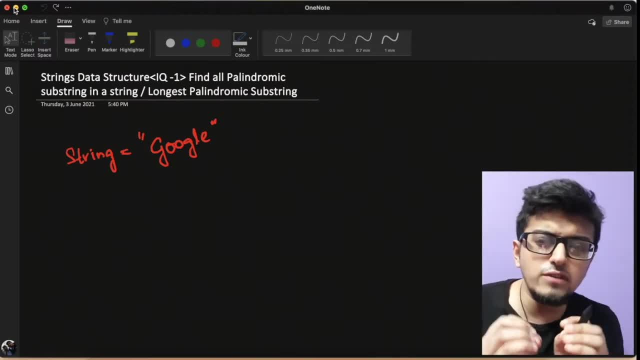 substring. so over here, if you carefully notice, both of the question is actually different. one is talking about finding all the palindromic substring within a string and the next question is telling about find the longest palindromic substring within that string. but the fun fact is the solution of both the problem. 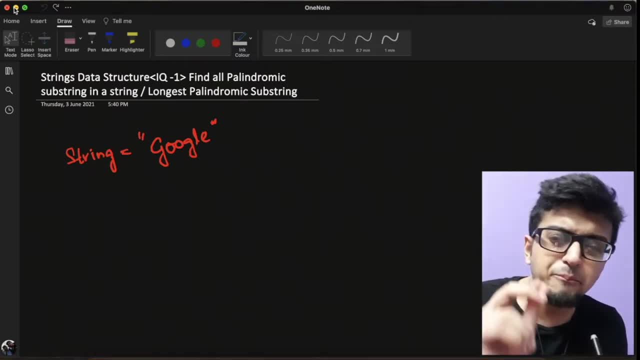 is more or less same. just by changing the solution a bit, we can actually get both the solution over here and in this way, at the end of the video I will be giving you the rest three problem that you can also solve with the help of this similar solution. so, without wasting much time, let's first understand the problem. 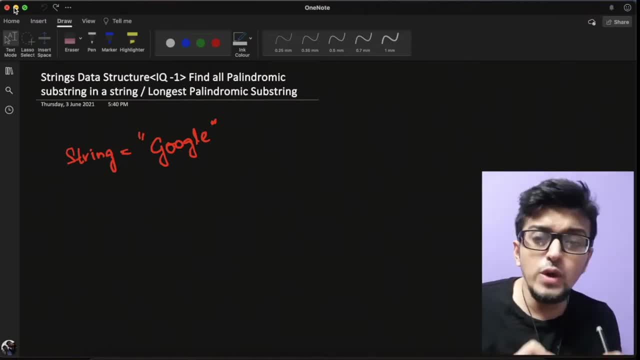 and let's see how, with the help of a single solution, we can easily solve so many problems during our technical interview. so let's first solve the problem of finding all the palindromic substring within a string. so let's first understand that. what is a substring? so a substring of a string is defined as a part of the. 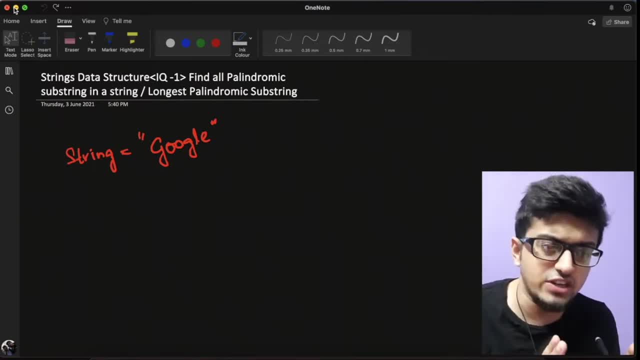 string in which all the characters are contiguous to each other. so over here within the string string google, you can see that the string that is g double o or g o, which align contiguous to each other, are actually substring, which means that if i try to write all the substrings, 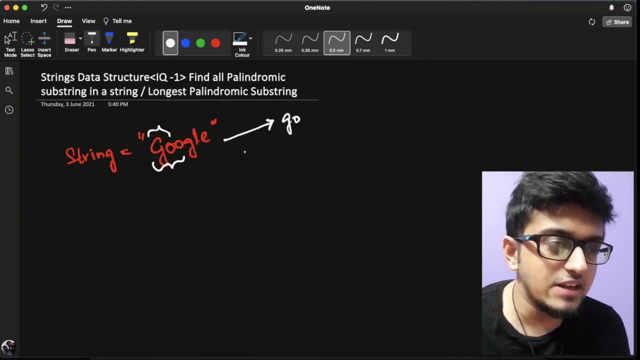 over here. g? o will be a substring. similarly, g double o will be a substring. g double o- g is also a substring, and in this way there can be plenty more substring over here. but one thing you have to remember: that all the characters within this substring should lie. 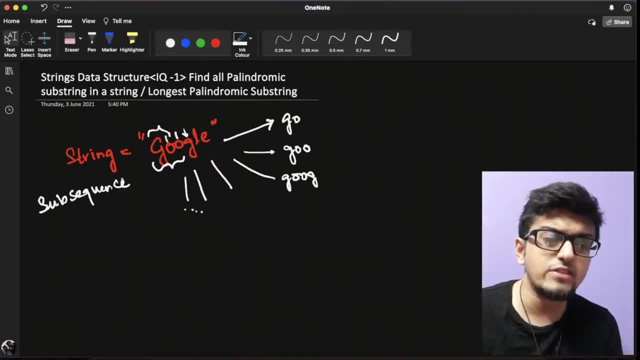 one after the another, whereas in case of the subsequence, which is another variety of a string, over there, the definition of the substring is: it is a part of the string, but it is not necessary that the character of the string will be contiguous to each other, which means: 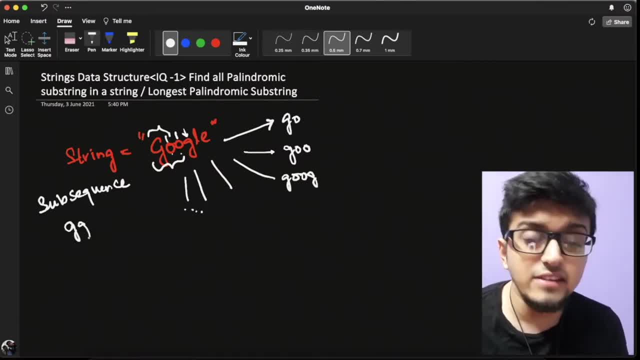 over here, g, g, le can be a subsequence. so over here you can see the first g is lying somewhere over here, the second g is lying somewhere over here, and so on. so over here, within this subsequence, all the characters of this subsequence are not necessary to be contiguous to each other. 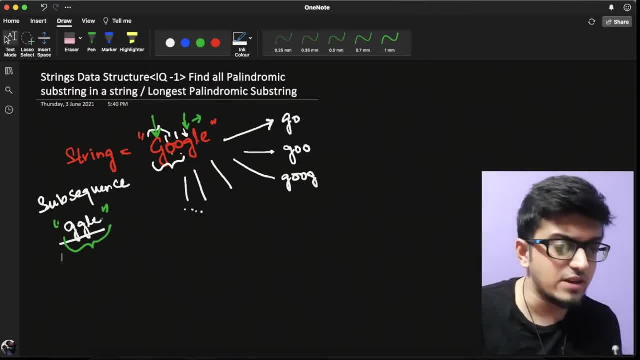 so this is the main difference between the substring and the subsequence. so over here now, if you see, the problem statement is telling that we need to find out all the palindromic substring within the string. so if we try to break down this problem into sub problem, the 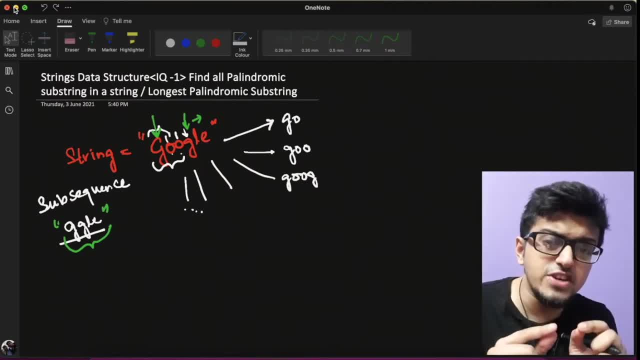 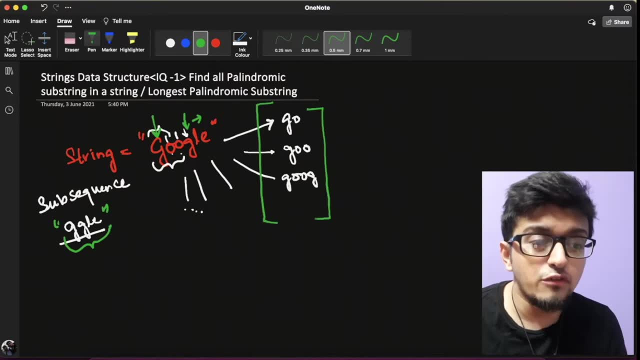 first problem statement is: the problem statement is: we need to find out all the substrings that can be generated from the string, which means that we need to find out this set of substrings which can be produced from this given string, over here and within this set of substring. we need to find out. 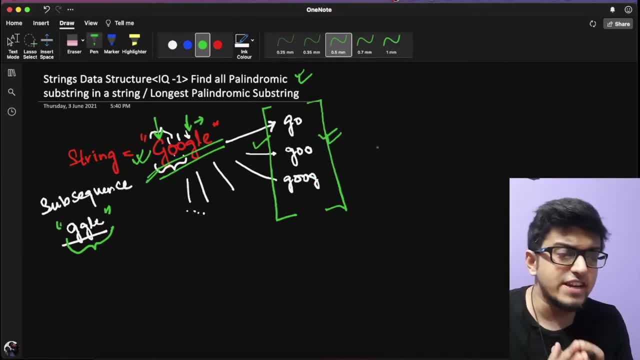 the parindromic substring over here. so a paringramic string is nothing but a string which is equal from both sides. so over here here, if we consider this string that is g falt, g falt. so you can see that if we divide this string into half, this string will be equal from this string. 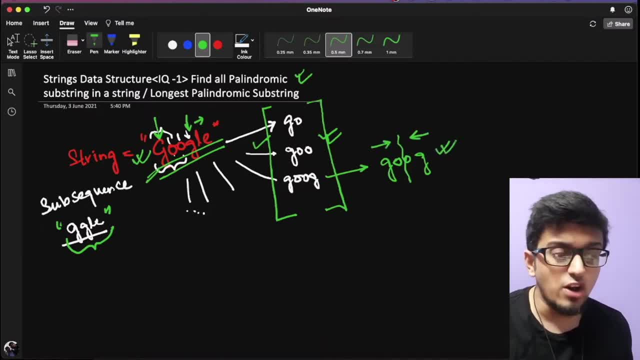 from both the ends. So this is basically the definition of a palindromic string. So in this way, after finding all the substring from a given string, we need to find out all the substring over here which are palindromic in nature. So over here, after generating all the substring that can be, 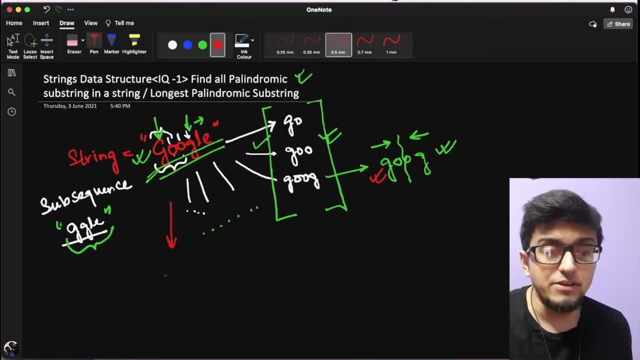 formed. you can see that the two palindromic substring that can be found over here are number one double O and number two G double O G. So these are the two palindromic substring that you can find out from this string. So I think this is clear to you. So the first problem statement is that 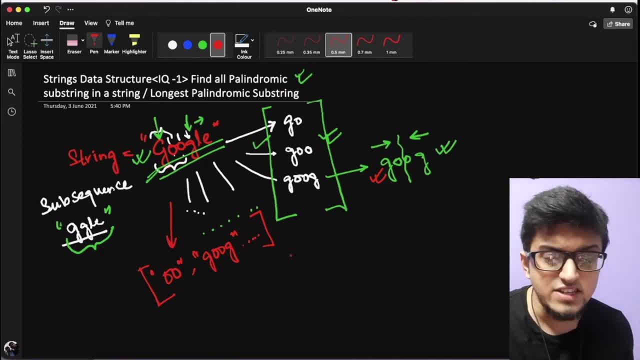 we need to find out all these substring which are palindromic in nature. and the second question is that we need to find out the longest palindromic substring over here, So you can see that over here, within this set of palindromic substring, this substring that is G, double O, G. 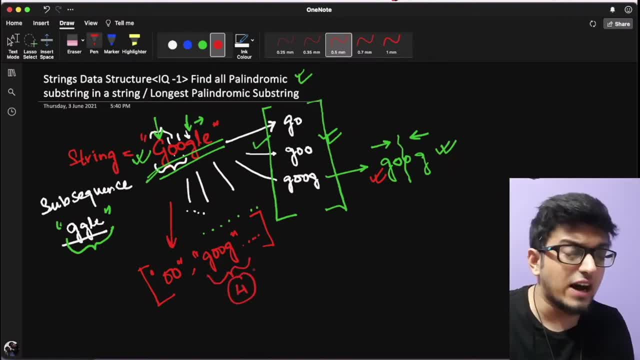 is the longest palindromic substring. So normally if you go to the other solution for solving the longest palindromic substring, you will find out that the most of the solution talks about the dynamic way of solving the problem. So I hope you know that. what is the dynamic program? So over 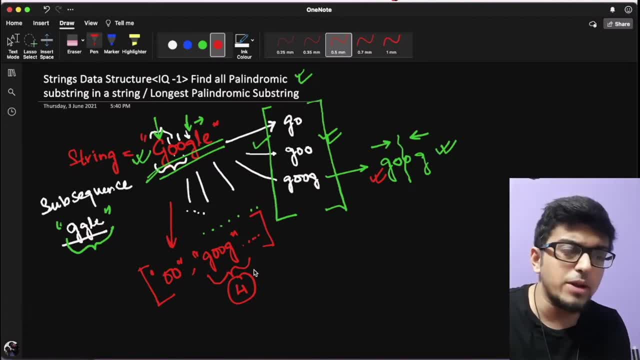 there. most of the solution tells that how you can solve this problem in a dynamic way. But very frankly, telling dynamic programming is a bit complicated if you do not know or understand the entire program. So to avoid the dynamic programming solution, you need to find out. 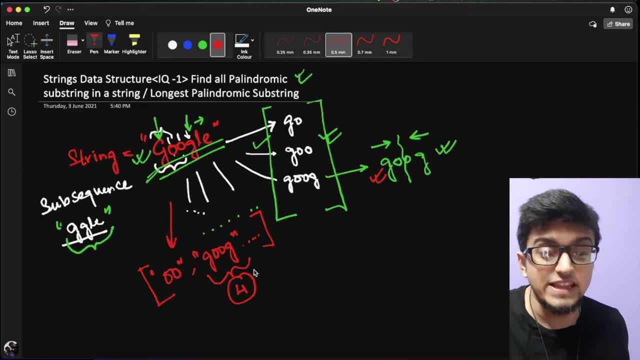 the solution for this problem. you can actually go with this solution that I will be providing over here, because the way we will be solving this problem will be very easy and you will see that you can easily remember and you can do it during your actual interview. So, without wasting much, 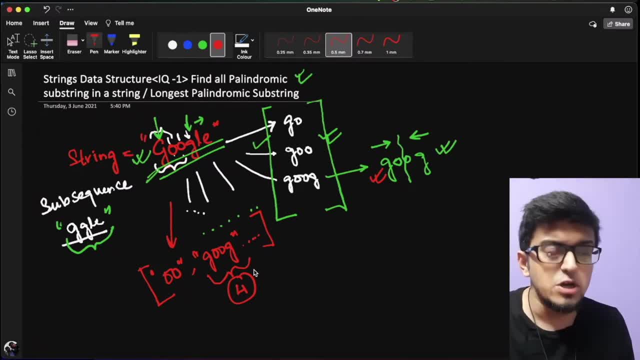 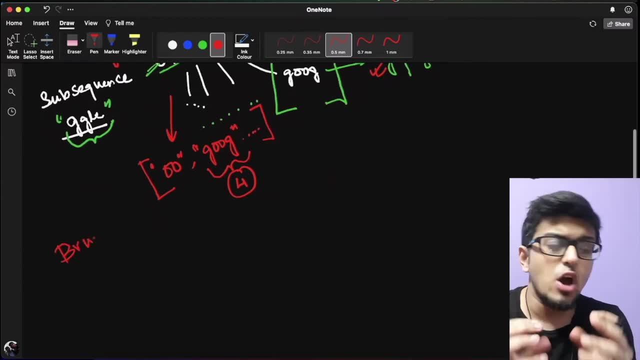 time. let's first discuss that: how we are planning to solve this problem. So, for the first time, we will go with the brute force approach, so that it will be easy for you to understand the basic solution or the basic way how we are planning to solve. So let's go with the brute force approach. 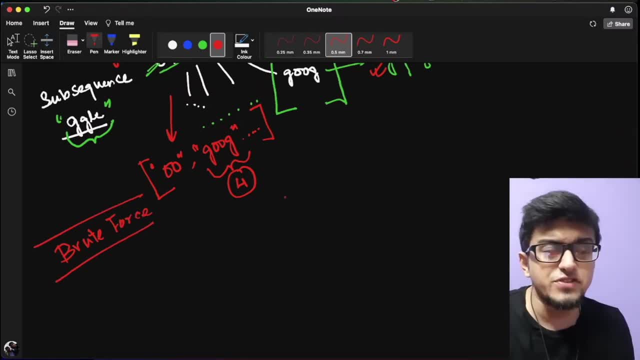 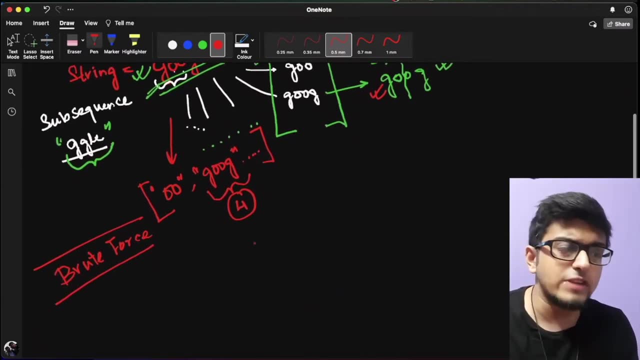 of solving this problem, that is, finding all the palindromic substring within a string and also finding the longest palindromic substring within that string. So let's start with the brute force approach over here. So the brute force approach of solving this. 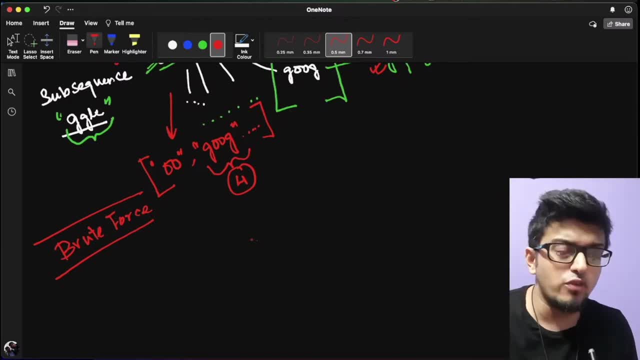 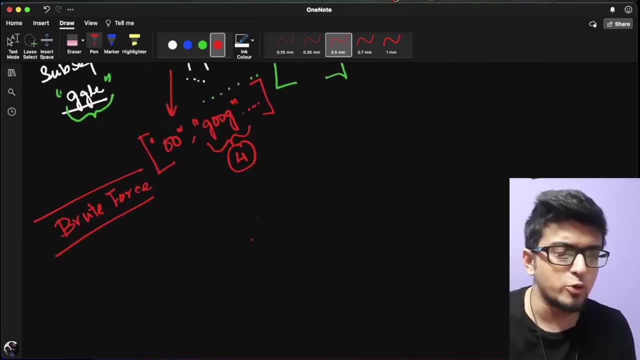 palindromic substring is pretty easy and straightforward, but over there there is one issue and that is complexity. So let's first see how we will solve the problem using the brute force approach. So, to solve the problem using the brute force approach, we will be going to: 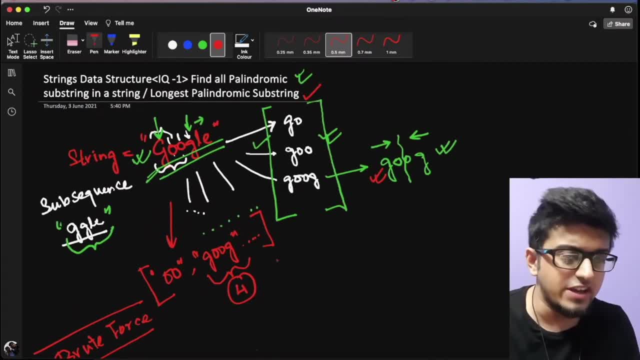 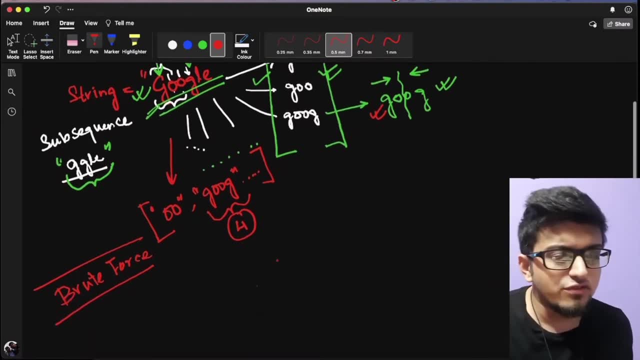 with finding all the substring that can be generated over here, and for that, to generate the substring from a given string, we will be using two for loop, So let's first write the two for loop that will help us to generate all the substring from a given string. 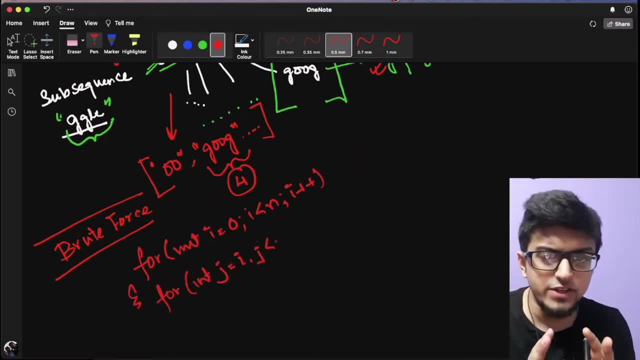 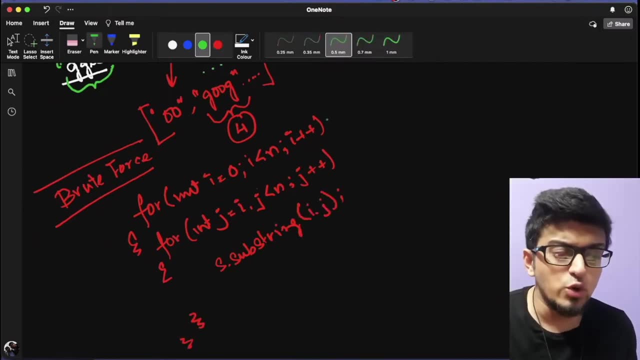 So over here I've just written the pseudocode, or the basic logic of this program so that it will be easy for you to code in any language. So over here you can see I have started two loops: one for loop starting from i, equal to zero, and another for loop starting from j equal to i. 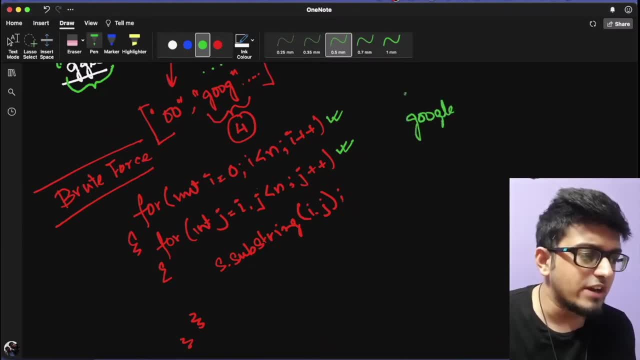 So what actually happening over here is like, for example, over here for the string google, we are starting two loops: one starting with the first index, that is, i, over here, and another starting with j, which is also pointing to i for the first time, and over here, if you. 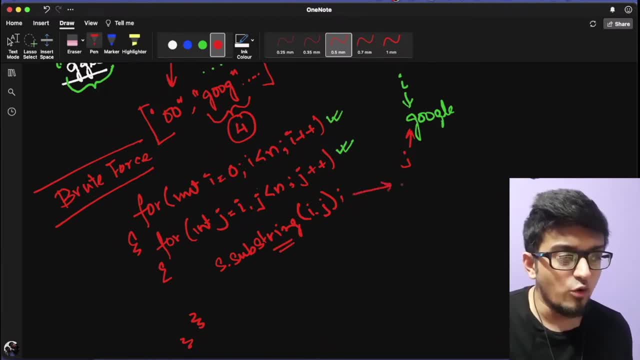 see the substring of i, j is nothing but g over here. So if you see over here, g- that is a single character of the string- is also a substring of a given string. and also, if you see, this is a palindromic substring because a single character of a string is. 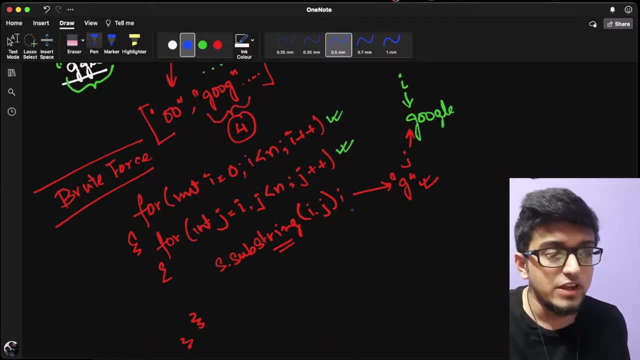 obviously a palindromic integer because it is always equal from the both side. So right now over here, if you see, there can be multiple substring that can be generated from here. So each and every character of this string is basically a substring, which are palindromic. 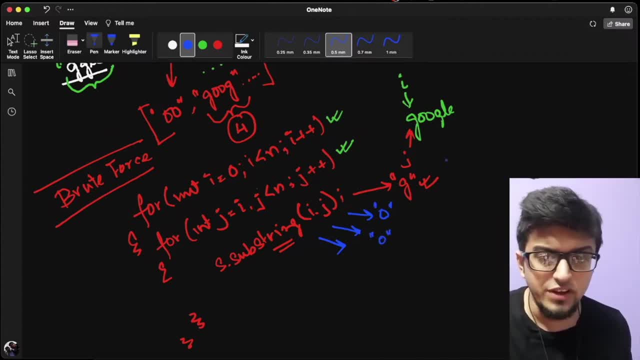 integer. So let's see how we are solving this problem over here. So this problem will actually calculate all the substring that are possible to be generated from this given string. So for the first time it will point to i equal to zero and j equal to zero, which means that 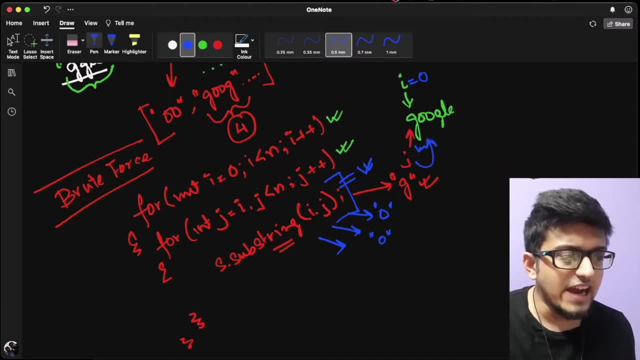 our substring that we will be producing will be g. On the second iteration over here, that is, when j will increase by one, the j will actually point to this index. that is, j will point to one and over here this substring will result into g. And in this way, as long as we increase the value of the g over here, you can see that. 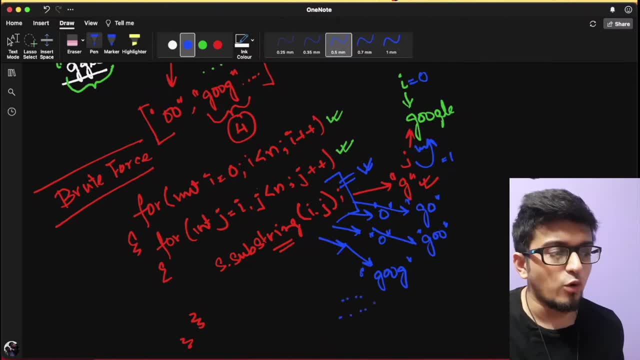 the substring will keep on generating something like this and so on. So in this way it will keep on generating the substring and on the next iteration, when the value of i will become one, at that time iteration will begin from here, which means that the first substring that will get generated for i equal to one, is o, and after that it. 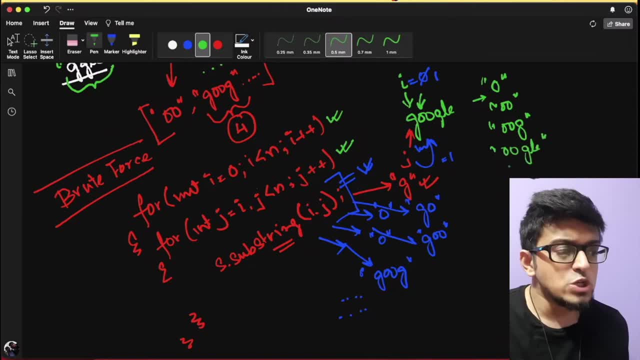 will be double o, then double o g, and so on. So this is the first substring that will get generated, for i equal to one is o, and after that it will be double o g, and so on. So in this way, on each and every iteration, we are actually generating all the substring. 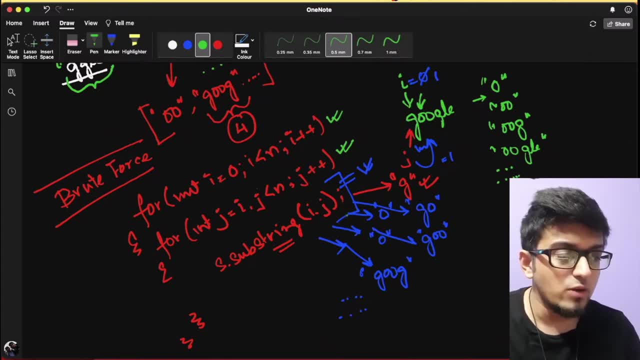 over here. Now the problem statement tells that we need to find out the palindromic substring over here, which means that over here we need to put one condition, and that is, we have to check that if this substring which is getting generated from here is palindromic or not, and if this 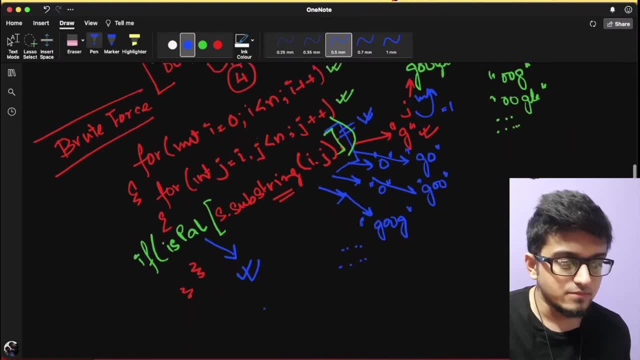 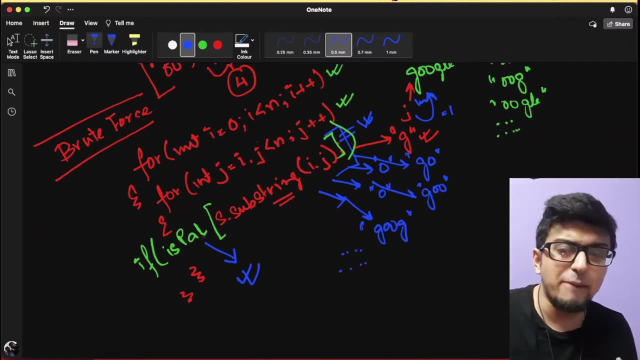 function that is isPalindrome, returns true, then we can predict that if this substring is palindromic in nature. So I hope this is clear to you, because this is quite a simple approach of solving this problem and if you just calculate the complexity of this program, you will see that the complexity 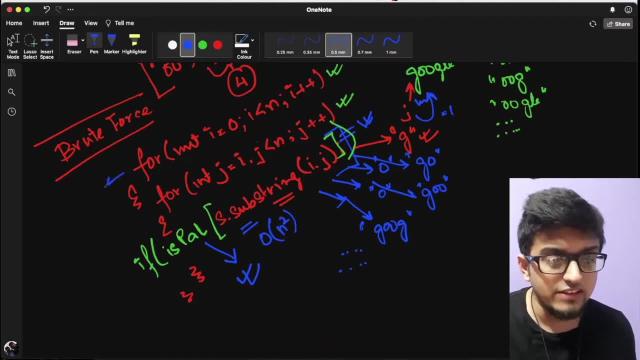 of finding all the substring. over here is order of n square. since we are iterating two times over here using an inner for loop, and over here to find whether a string is palindrome or not. we are using another functionality that is isPalindrome and you know that the complexity 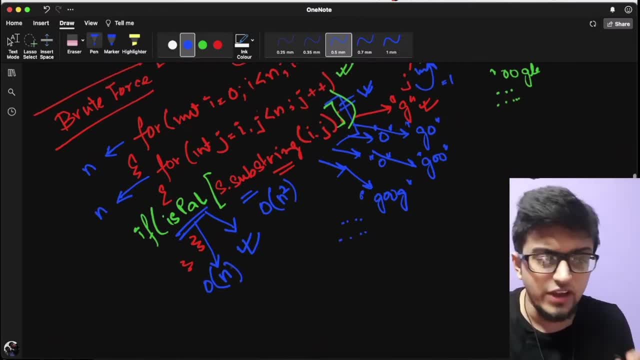 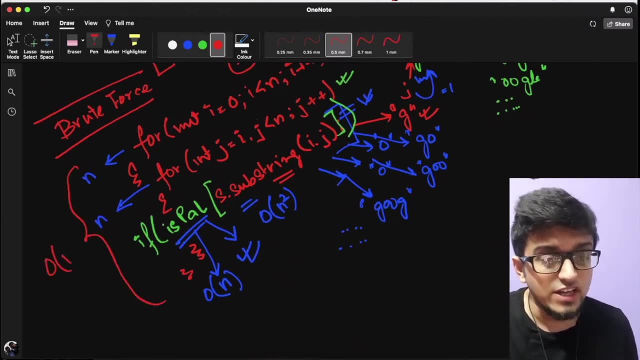 to find a string as a palindrome or not is order of n, which means that the complexity of this function will be order of n and the overall complexity of this problem will be order of n, cube, which is actually quite high for the real time scenario. So over here we need to find out a better solution which can result into a less complex 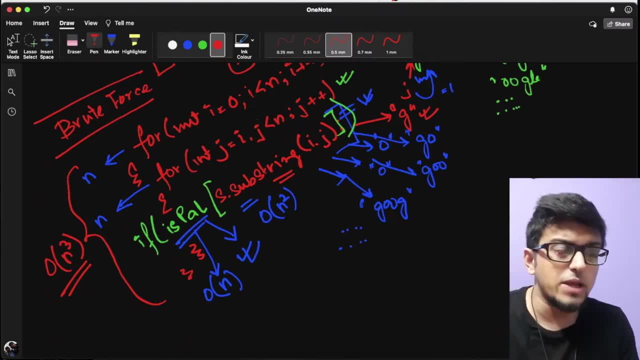 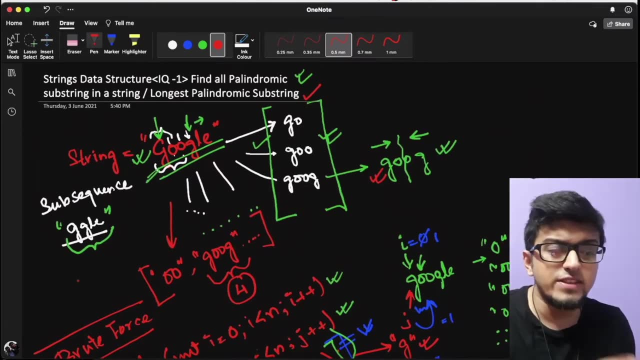 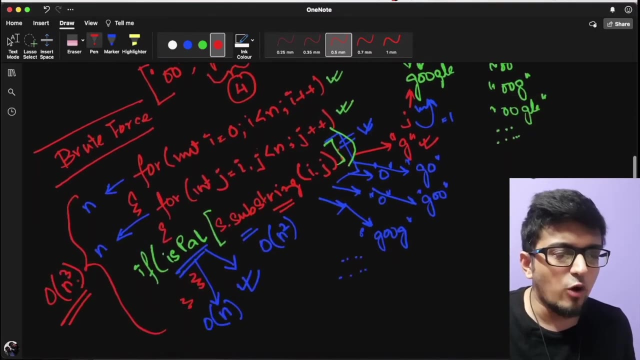 algorithm. So let's see how we can solve this problem using some other algorithm which will result into an optimal solution. So I hope you guys are clear with this basic solution that how we are solving this problem using the brute force method. So over here you can also see that you can also calculate the longest palindromic substring. 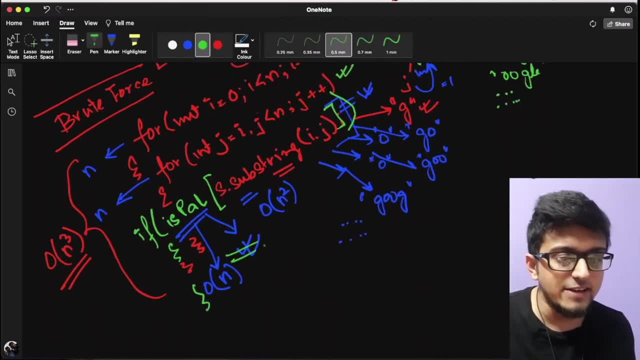 from here by just putting another condition within this, if block, that if the palindrome is a substring, then you have to again put a check that whether the length of that palindromic substring is greater or not. So just by putting one more condition over here you can easily get the result. 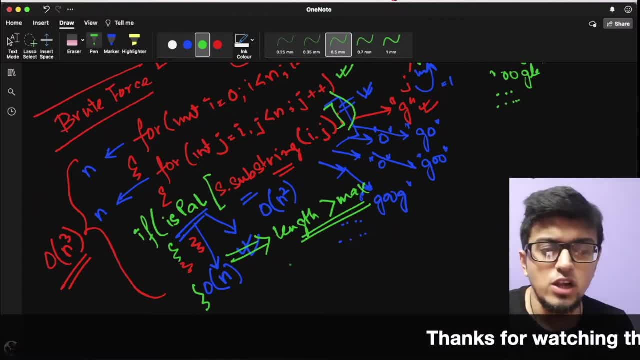 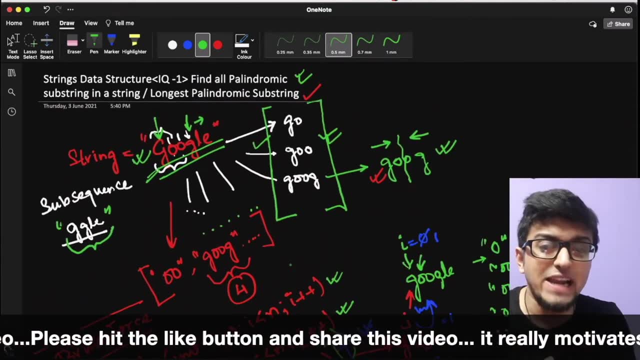 So I hope you guys are clear with this basic solution that how we are solving this problem using some other algorithm which can result into a less complex algorithm which can easily get the result over here for the longest palindromic substring. So I hope right now you got the idea that why I am telling that all this problem on 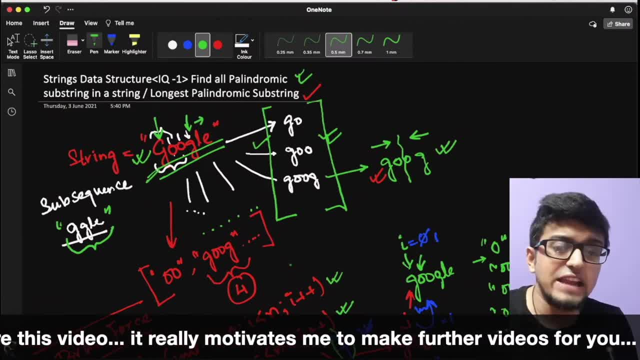 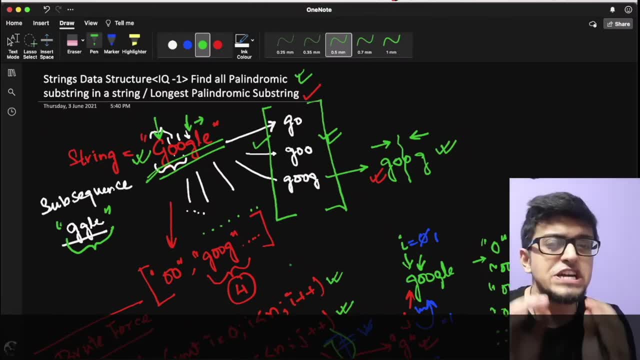 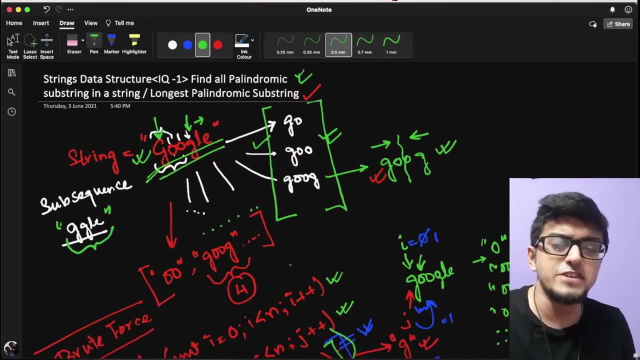 palindromic substring are interrelated with each other and if you know the solution of only one program, you can actually solve all the problems related to palindromic substring during your interview process. So, without wasting much time, let's start with understanding that how we will be solving. 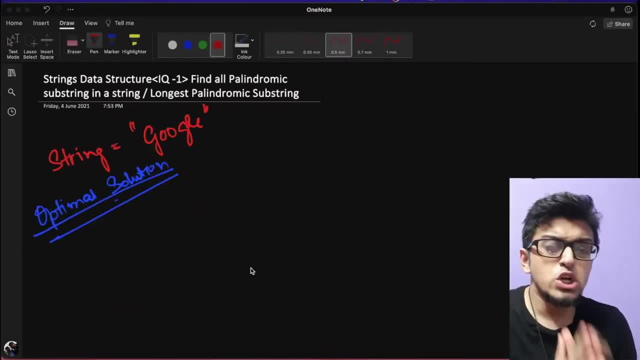 this problem using the optimized solution. So the way by which we will be solving this problem using the most optimal solution is pretty easy and straight forward. So you will notice that a string which is palindromic in nature can be of two types. 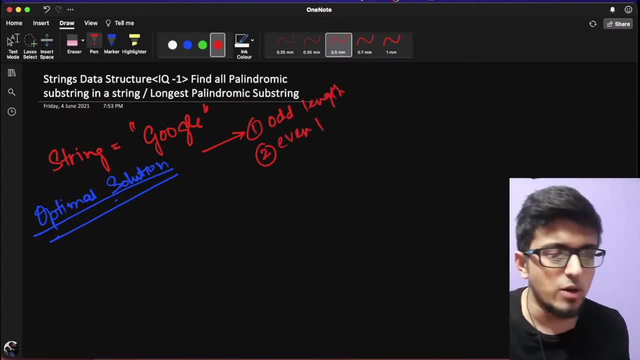 Number one is the odd palindrome and number two is the even palindrome. So if you just remember, I have just told that the substring of this string is nothing but each and every character over here. So G is one of the substring. Similarly, O is another substring. 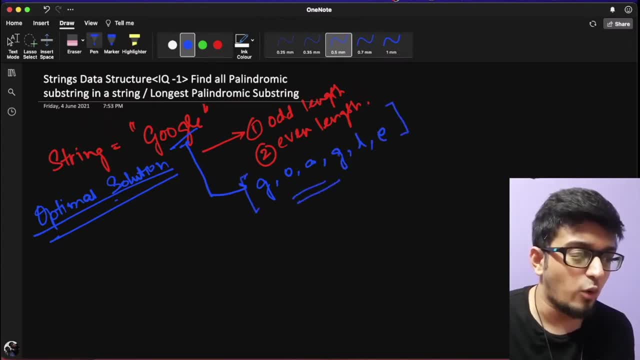 Again, O is another substring, then again comes G, L and so on. So over here, each and every string is a substring. and not only that, since a single character is a palindrome. that is why this is a single character, palindromic substring. So over here. if you just see, these are all the example of the palindromic substring. 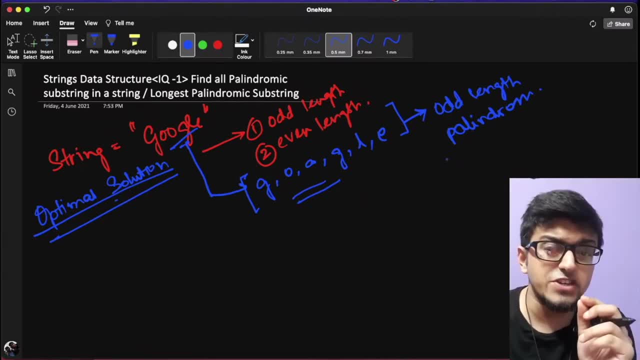 And if you just look at this carefully, these are all the palindromic substring of odd length, because the length of all the substring over here are odd, So I will mark this as odd palindrome. Now, the next set of palindrome or the next set of palindromic substring that you can see: 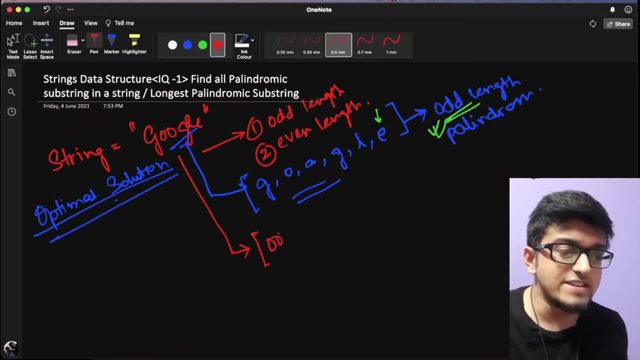 over here is double O, which is actually nothing but a even set of palindrome. So if you just think deeply, you can easily conclude that the palindromic substring within a string can be of two types. Number one is the odd palindrome and number two is the even palindrome, and this will be 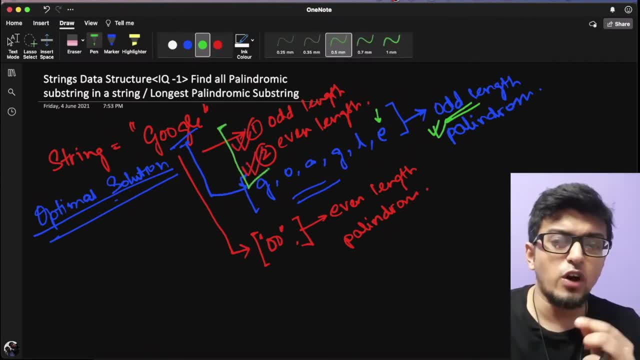 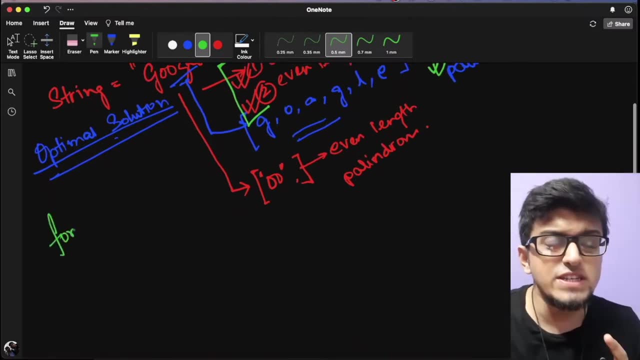 the point to solve the problem. So let's see how we will be solving this problem. So over here we will be running a follow from i equal to zero to i equal to n, which is the length of the string, and over here we will take each and every character as a special. 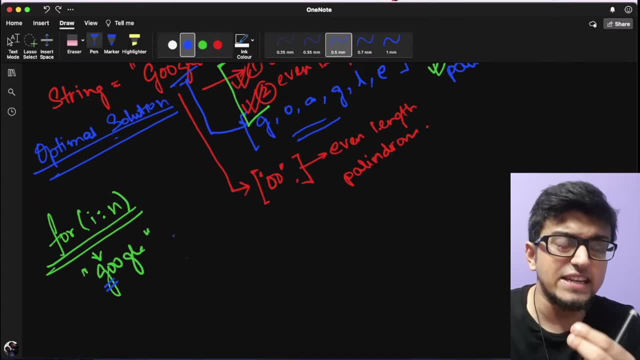 character, that is, we will consider each character as the middle character of the palindrome, which means that all the character which are lying beside it on the left side and the right side should be equal. So over here, If I take an example of a even length palindrome, let's consider a string that is pal lap. 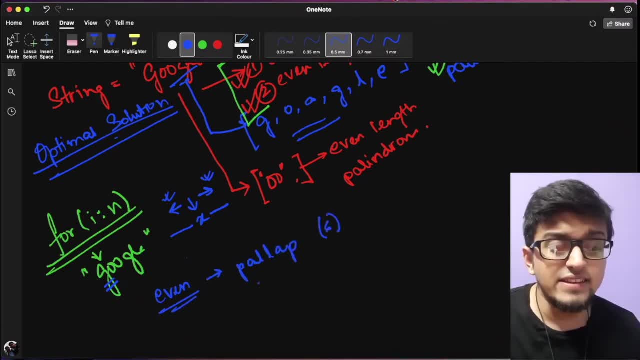 So you can see, this is a six character substring and this is a even length palindrome. and let's take another example of palindrome and that is pal ap. So obviously this words doesn't have any meaning, but let's, for the demonstration purpose, I'm taking all this example. 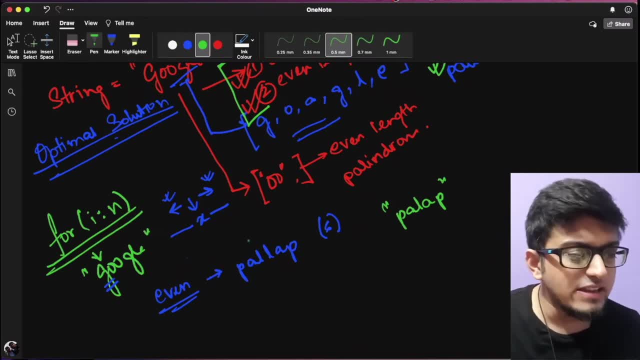 So let's see how we are planning to solve this problem. So over here, This is a odd length palindrome and over here what we will be doing it on each and every iteration on this string, we will be considering that the string on the character which we 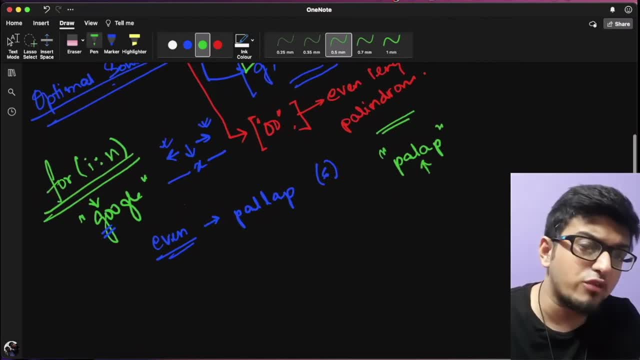 are getting for. the value of i is the middle character of the palindrome, For example, for i equal to two. over here for this string the pointer will be over here, right, because over here the caret function of i will result into the l, which is the middle. 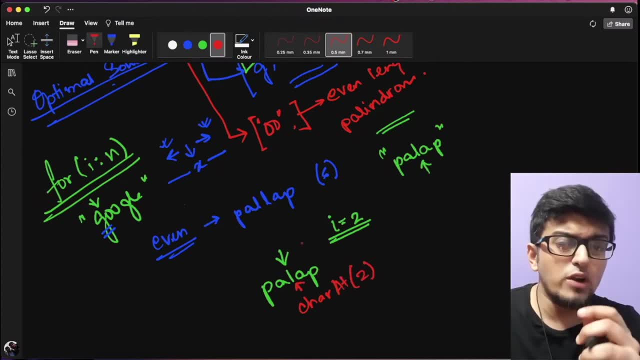 character over here. So I think that's it. I think this is clear to you. So what we will assume that on each and every iteration we are in the middle of our palindromic substring means if we go into our left or into our right, we will see the same character. 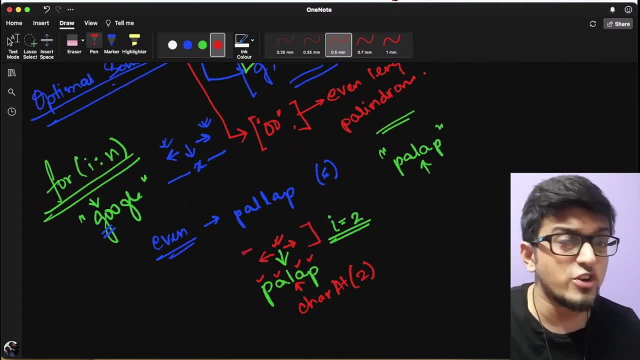 on both side, and we can easily conclude that this is a palindromic string. So over here you can see how, with this assumption, we are solving this problem. So I know, though, you can visualize this code, but the concept is still not clear to you. 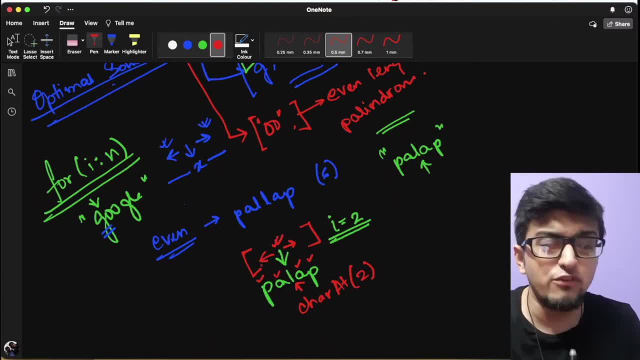 So let's now do our dry run over here, So that it will be helpful for you to visualize the complete code of how we are trying to find out the solution of this problem, and over here, if you just notice the complexity of this problem, will be nothing but order of n square. 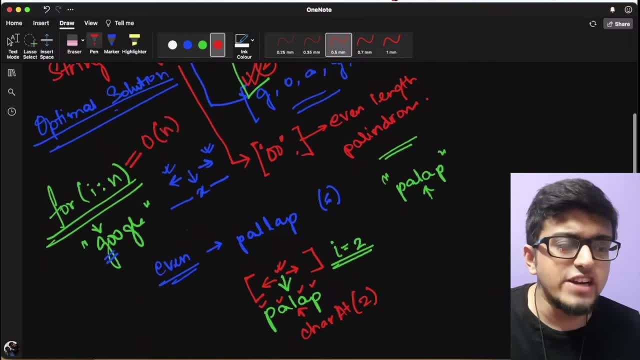 So here, if you see, we are using one for loop to iterate over each and every character over here. So for this we will be using one for loop that will run from i, equal to zero, to i equal to n, And over here to find out that, whether a string is palindromic or not, the complexity of these. 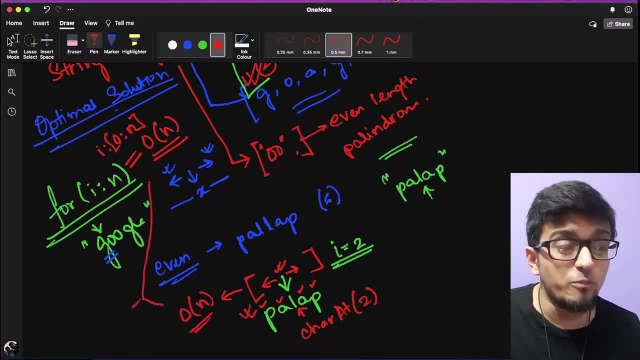 will be order of n, Which means that the entire complexity of this algorithm will be order of n? square. So I hope this is clear- how we are getting the order of n square complexity over here. Now, since you have understood that we are successful in reducing the complexity of the 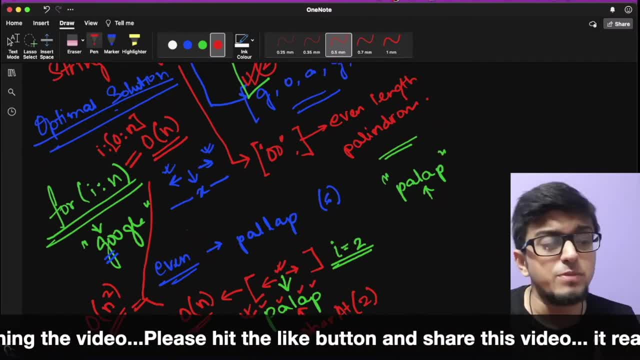 program. let's now understand the algorithm by which we will be solving this problem. And for that, as usual, we will begin our dry run over here. And for that, as usual, we will begin our dry run over here. And for that, as usual, we will begin our dry run over here. 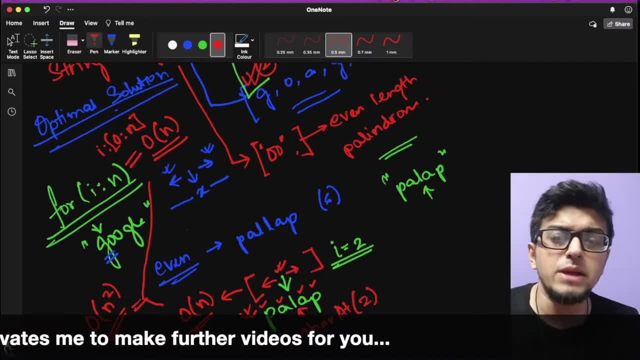 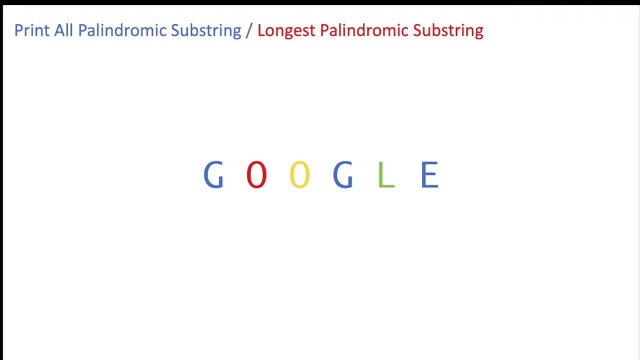 So let's start this program by using our visual display pool. So let's understand the problem using the Visual display Pool. So over here we will be solving both the problem together, That is, printing all the palindromic substring and also finding the longest palindromic substring. 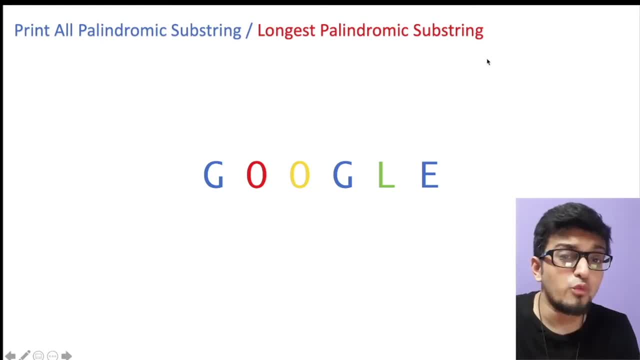 without the dynamic program. So let's see how we will be solving this problem. So to solve this program in the most optimized way, we need an additional data structure and that is a hash state. you know, a hash set is nothing but a simple data structure which are used to store any data type. 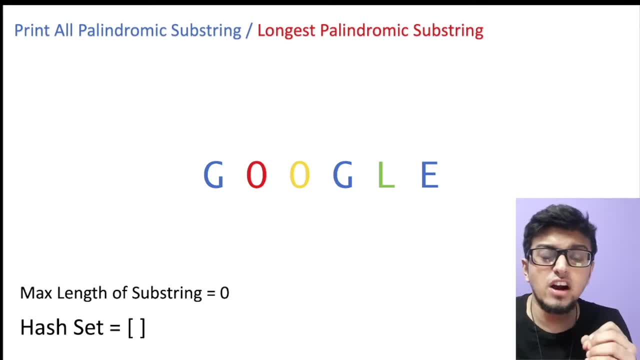 without any duplication, which means that a hash set doesn't contains any duplicate value within themselves, which means that if i insert two a within a hash set, it will only store a single a within itself. so over here, to solve this problem in the most simplest way, we will be using a asset. 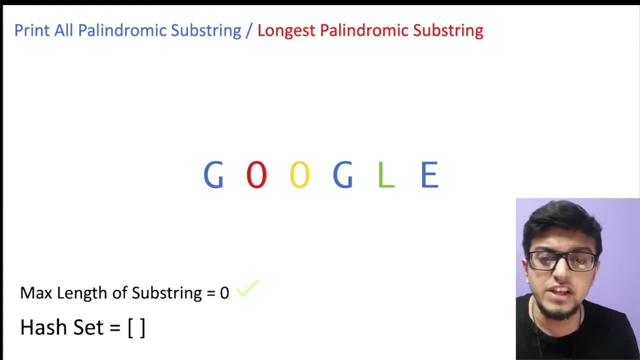 over here, and also we will be using an additional variable that will keep a counter of the length of the maximum substring that we have encountered until now. so let's see how we will be doing so. as i have already told you, we have two type of palindromic substring. one is the odd length. 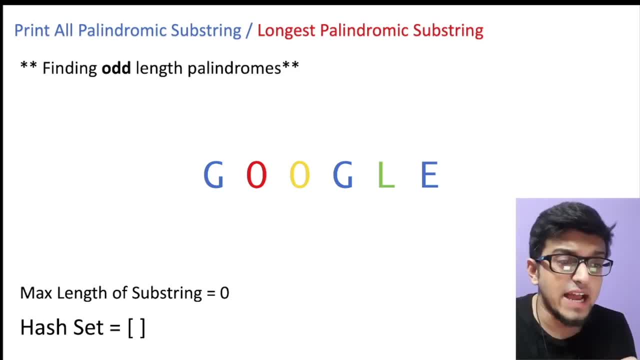 and another is the even length, and over here, for the first time, we will be finding all the odd length palindrome that can be found over here. so let's first calculate all the odd length palindrome over here. so we'll start our iteration from i equal to 0 and over here, if you see, for i equal to 0, the 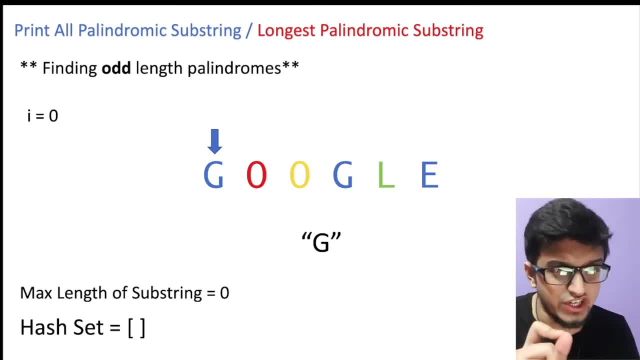 first character that we are encountering over here is g, and i have already told you that a single character is the example of both the palindrome as well as a substring. so over here, this character g satisfies both our condition of being a palindromic substring. so since over 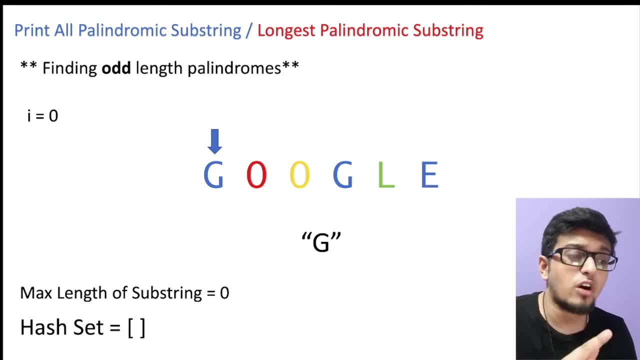 here we already got one answer of our problem, that is, we got the first palindrome, and that is why we will be storing this palindromic substring within our hash set and we will update the length of the maximum palindromic substring by one. so let's insert. 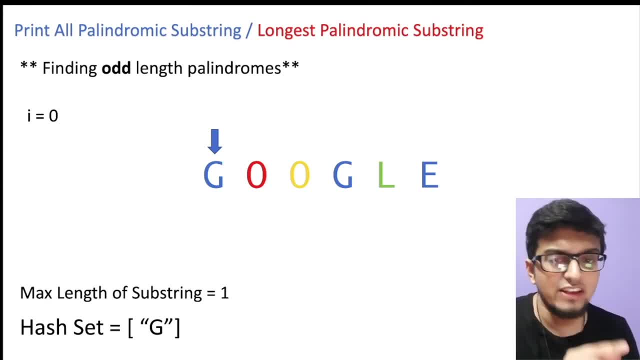 this g into our asset and let's update the value as one. now comes. the fun part now: what we have to do, since we are considering that, whatever the index which we are targeting, that is for i equal to 0. that is the middle of our palindrome, which means that all the characters which are lying on 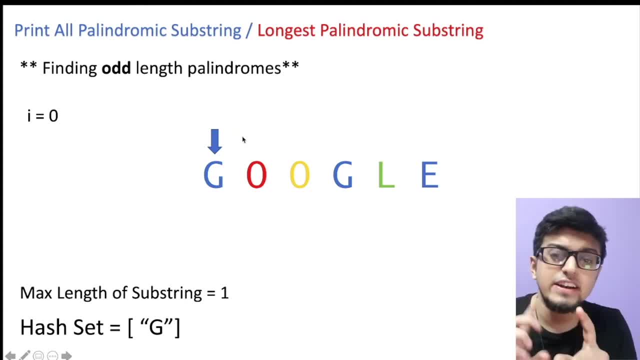 both sides of this character should be equal, otherwise it is not a palindromic substring. so we will see that, keeping g as a center point, that is the middle of the palindrome, how long we can increase the window size of our palindrome and we can check that, whether that substring is. 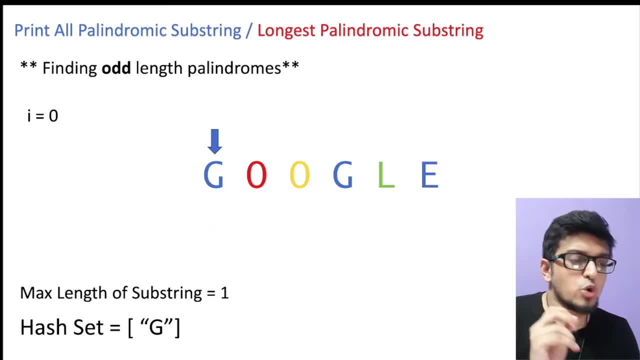 palindromic or not. so let's see what i mean to say. so over here you can see that the character which we have encountered is g, which is of size one. now, what we will do, we will say two point does from here, one going into the right side and one going into the left side, and on each and every, 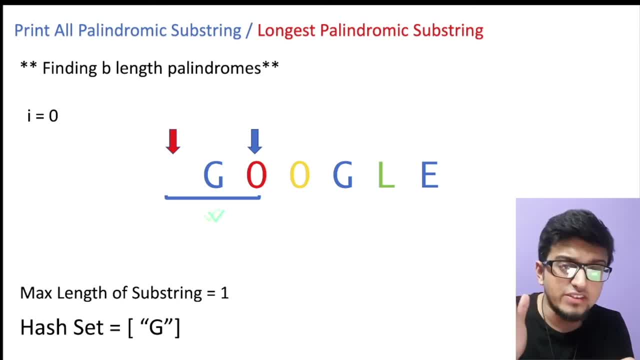 iteration, we have to check that whether the character on the left side is equal to the character on the right side and if this two character is equal, which means that the entire substring that we have got until now is palindrome, and otherwise that the substring that we are. 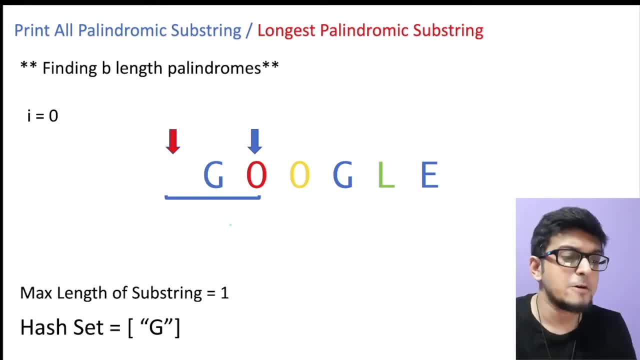 calculating right now is not a palindromic image, so let's see, with the help of this algorithm, how we are solving this problem. so, for the first time, you can see, we are increasing our window size to one. so over here, keeping g as our central point, we are increasing the window size over. 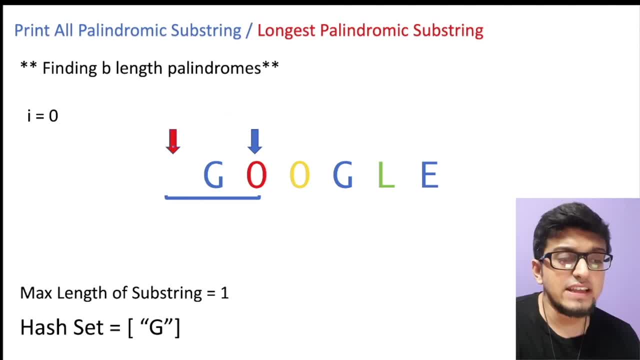 here with the help of the two pointer. but over here you can see that our left pointer, which is our low pointer, has already went outside our string boundary, so obviously we cannot take this substring into consideration. so we will stop the iteration over here and we will increase the. 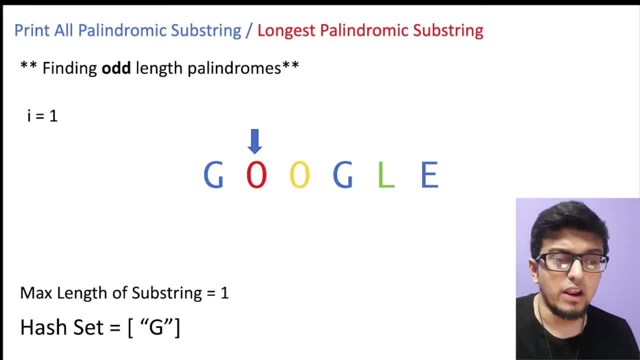 value of i. so let's increase the value of i equal to 1 and over. here the character that we have got is o and, as usual, o is a substring and also it is a palindromic in nature, so let's put this o into our. 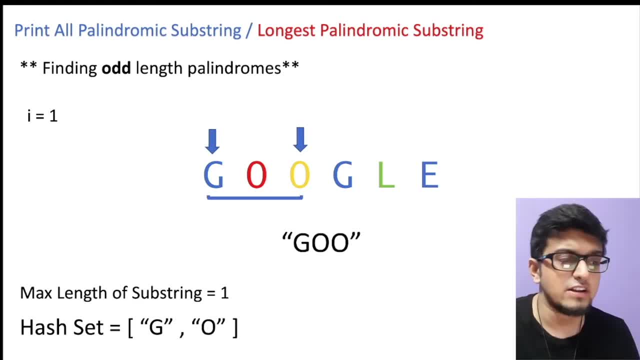 hash set and let's also increase the window size over here. so over here you can see the character which are within this window are also odd in length and since this substring is not a palindrome, there is no need of increasing the window size over here, because any substring that will be having g, double o inside it, which is not a palindrome. 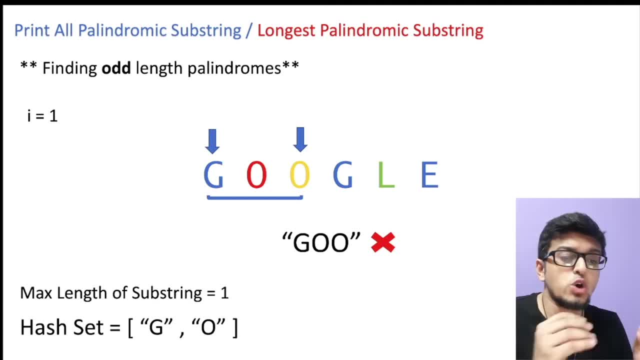 will also result in a non-palindromic substring. so we will again stop the iteration over here and we will increase our pointer to i equal to 2.. now, over here you can see, o is another palindrome over here, which is a substring, and over here, since o is already in our hash set. so even though if we 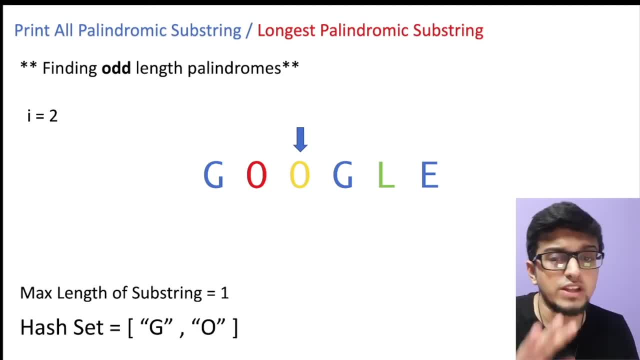 insert o into our hash set, it will not result any change within our hash set, because hash set doesn't contain any duplicate element within itself. so the hash set will remain same and the palindromic substring that we had encountered until now will be g and o, and in this way we will keep on proceeding so over here, since o is a. 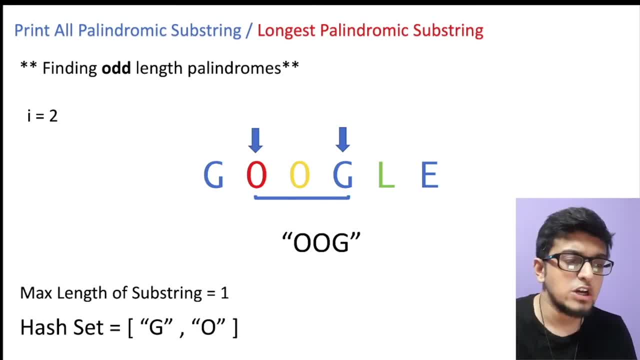 palindromic substring, we again have to increase the window size. so again, we will increase the window size and we will see that the substring we are generating is double o, g, which is again not a palindrome, which means that we will break this iteration and we will increase the pointer. 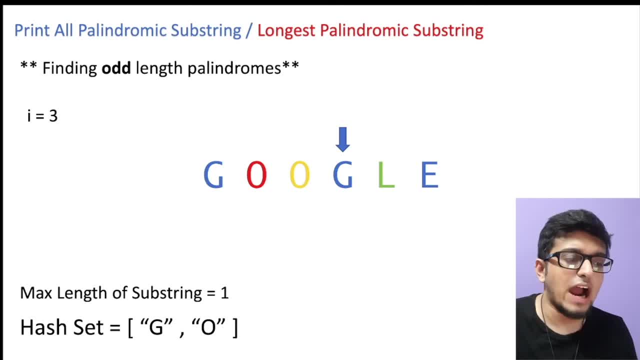 to i, equal to 3, and in this way we will keep on iterating forward. So I hope this is clear to you. until this point, and over here, you can see, since on our last case the pointer is going out of range of our string boundary, so we have to stop our iteration over here, and thus we can conclude that. 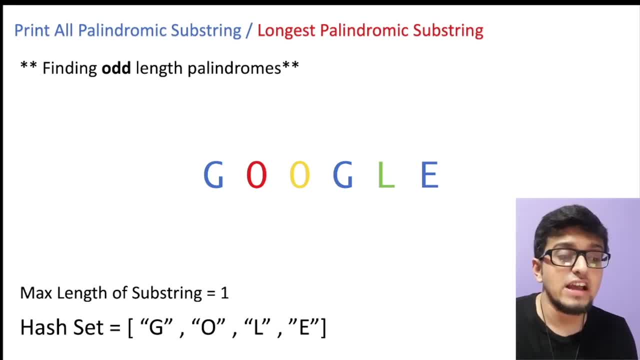 these are all the odd-lane palindrome which can be generated from this given string, that is, google. Now let's see how we will be finding the even-lane palindrome over here. and obviously, to find out a even-lane palindrome, we have to consider a window size of 2.. Thus we will be making a window. 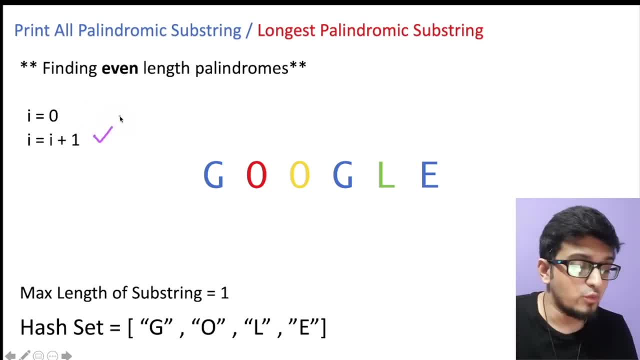 size from i equal to 0 to i equal to i plus 1, which is this 2.. So, for the first iteration, we are having a window size of 2, which is, though, a substring, but this is not a palindromic substring. 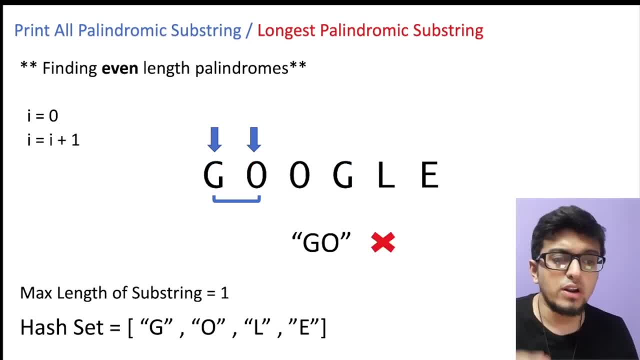 So what we will do, we will stop our iteration and we will move forward with i equal to 1, and this time you can see that the substring that we are encountering is double o. and here comes a fun fact of how we will be finding the palindrome. 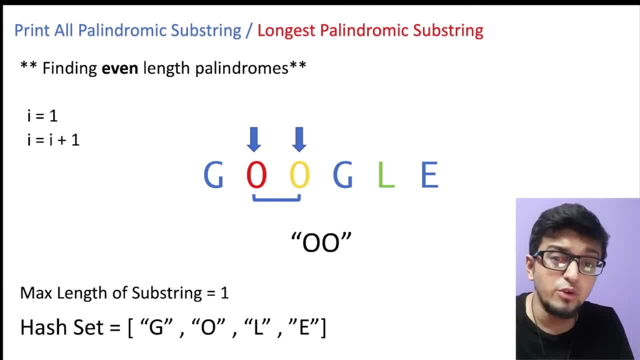 because with the help of this example you can see how easily we are checking the palindromic substring over here. So over here, for the first case, over here you can see double o is our palindromic substring, and since this is a palindromic substring, we are blindly putting the value. 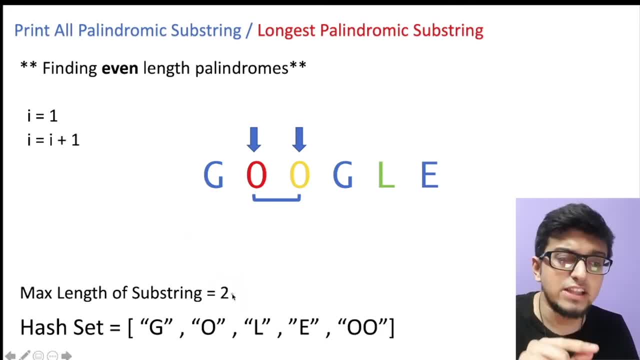 of the palindromic substring over here. So over here for the first case over here you can see that we are putting the value of the palindromic substring over here and we are also increasing the maximum length of our palindromic substring to 2, because until now double o is the maximum. 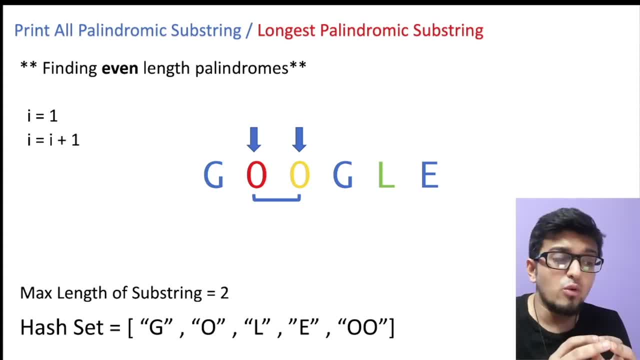 palindromic length that we have encountered over here Now, over here within this algorithm, since we are considering that the character which are under consideration are the middle part of our palindrome, which means that all the character beside that middle part should also be equal, and if it is equal, we will also consider that as one of the palindromic substring. 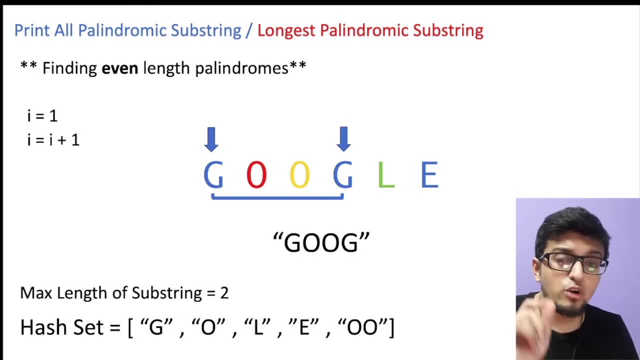 And thus what we will do. we will be increase our window size and thus the substring which we are getting is g, double o, g and over here. if you look carefully, this is also a substring which is palindromic in nature, and thus we will be also putting this value into our hashing and also we 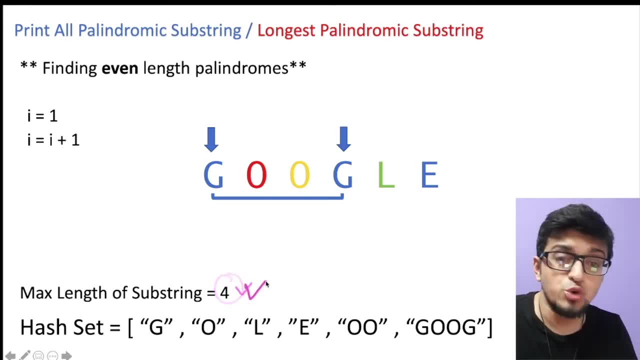 will be updating the maximum length of the palindromic substring to 4.. So you can see how easily we have solved this problem of finding the maximum length of the palindromic substring to 4.. Now let's move forward with the iteration. So what we will do again over here, since this is a palindrome. 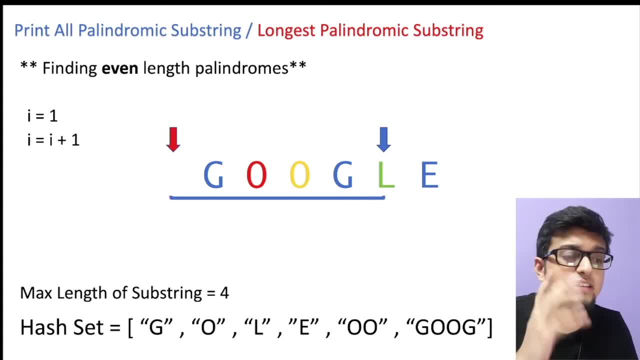 we will again increase the window size over here, but in this case the left hand side pointer moved out of our index size, so we will stop over here and we will increase the value of i due to and. in this way we will keep on moving forward and we will check on each and every iteration that, whether 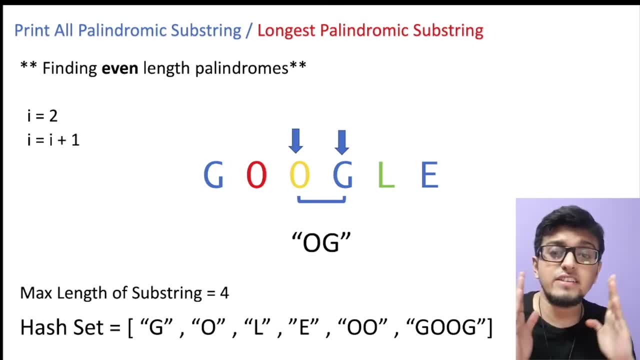 palindromic or not. and if it is a palindrome, then what we are doing we are increasing the window size and we are further checking that whether that string which we got after increasing the window size is also palindrome or not. and in this way we will complete the entire iteration from i equal to 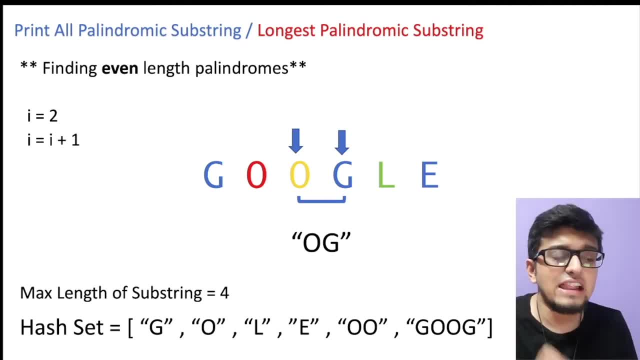 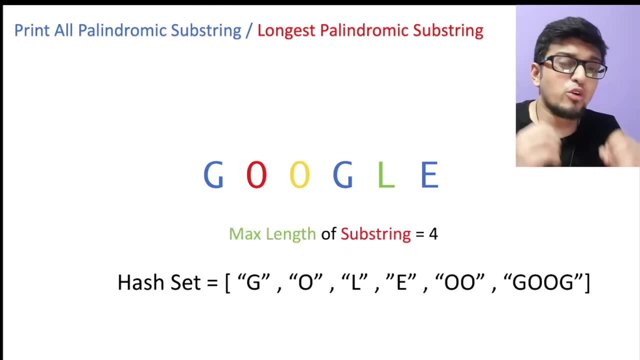 0 to i, equal to n. So let's proceed further over here and let's see how the other values are getting calculated over here, and thus, over here we reached the end of our string and we have completed the entire check of finding the palindromic substring. and over here you can see. 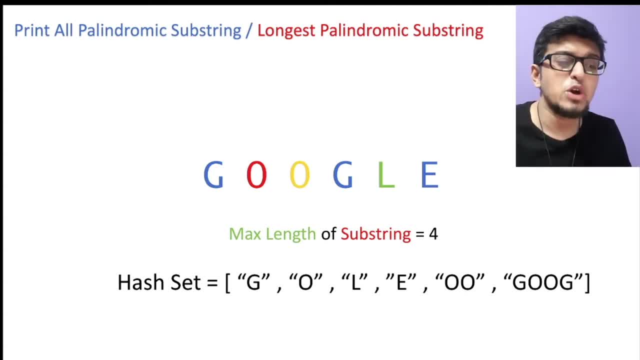 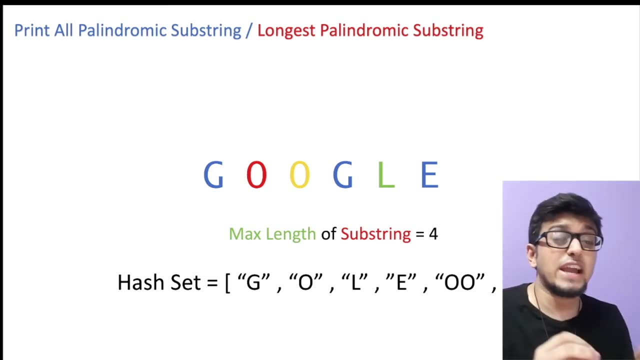 how easily, after the end of the entire iteration, we have calculated all the palindromic substring that can be generated from this given string, and from here also we have found out the maximum length of the palindromic substring over here. So you have seen that with the help of this simple 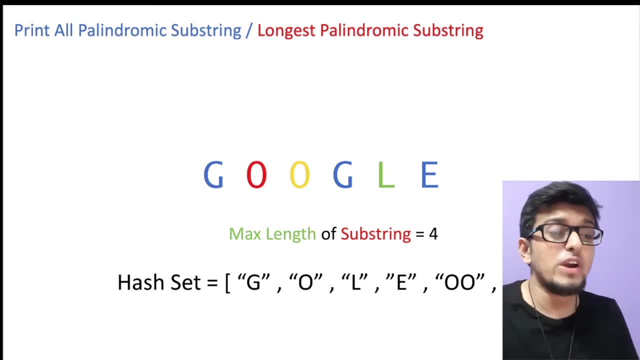 algorithm how easily and how efficiently we have solved both the problems over here. So hopefully this video was useful to you to understand that how we are solving this palindromic substring problem. and if you have liked this video, do not forget to like and share. 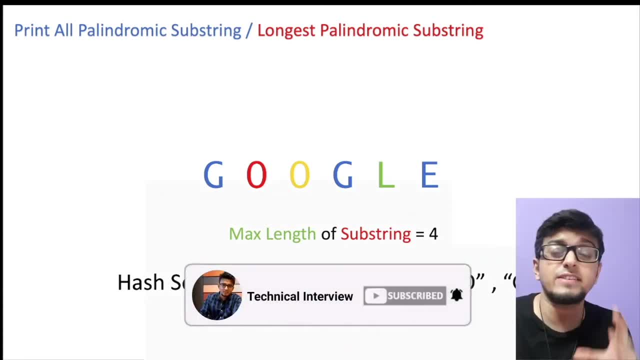 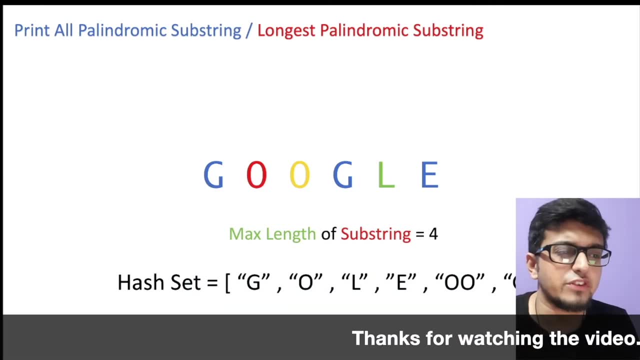 this video and if you are new to my channel, do not forget to hit the subscribe button and hit the bell icon so that you never miss an update from my site and you are always ready for your next interview. So, without wasting much time, let's see how we will. 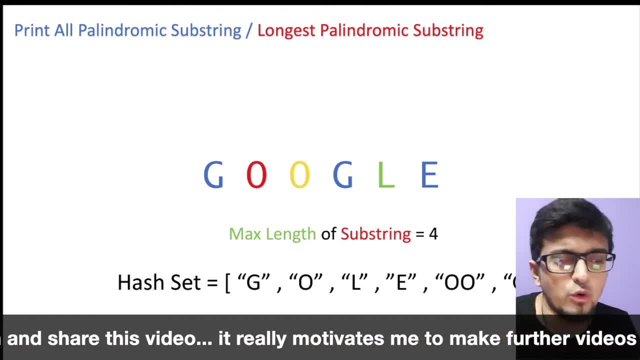 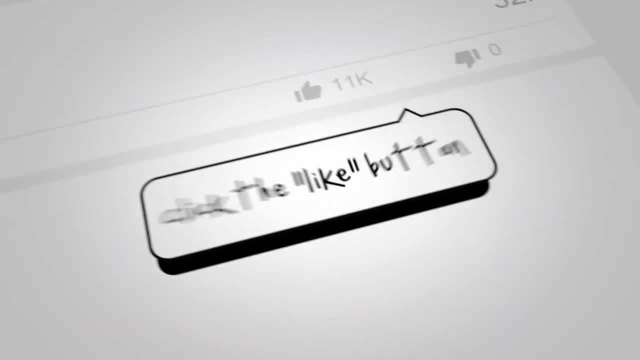 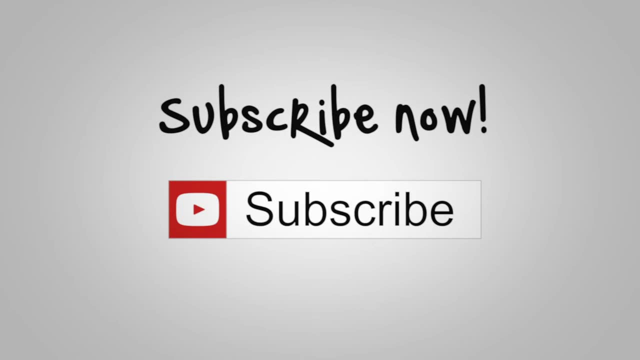 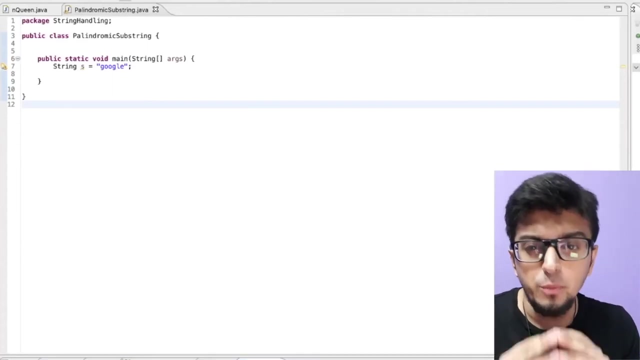 be implementing the entire algorithm using our java code. So let's go with the implementation of this entire algorithm using the java code. So now, since you guys have understood the algorithm by which we are solving this problem in the most optimized way, let's now implement the algorithm over here. and over here you can see to. 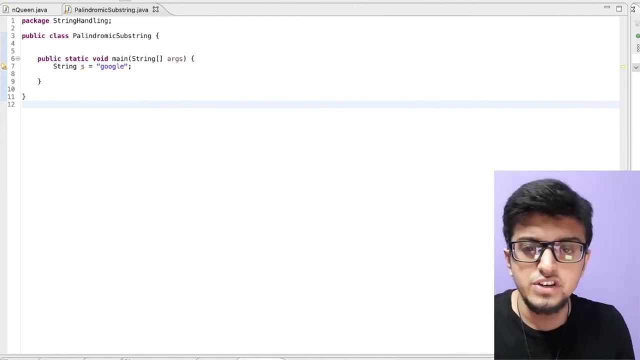 implement the algorithm of finding the longest palindromic substring. I have created a class called as palindromic substring And within this there is a string called as google. So over here, the way we will be implementing the algorithm is quite simple and basic. So over here, let's write a function. 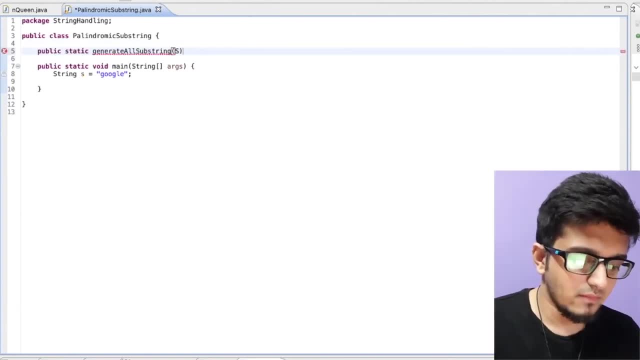 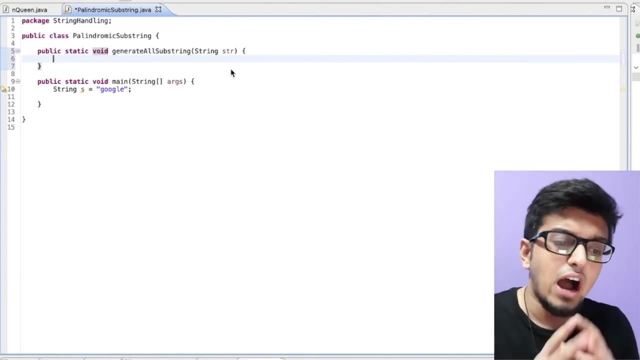 called as generateAllSubstring, and within this function we will be writing the logic of generating all the substring that can be driven out of a particular string. So let's call this function from here. Now, since we have called our function, that is, generateAllSubstring from our. 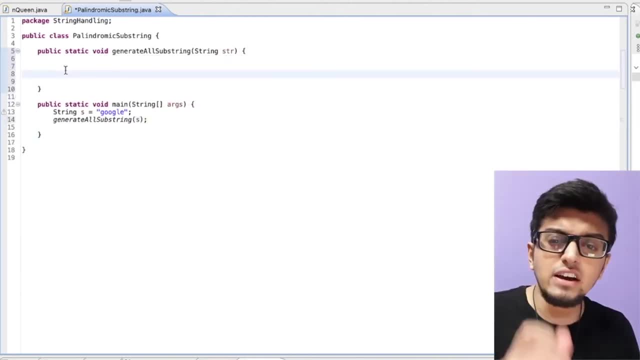 main block. Let's write the logic over here. So, as I have already told you over here, we will be running a for loop starting from i equal to 0, to i equal to n, which is the length of the string. So let's write. 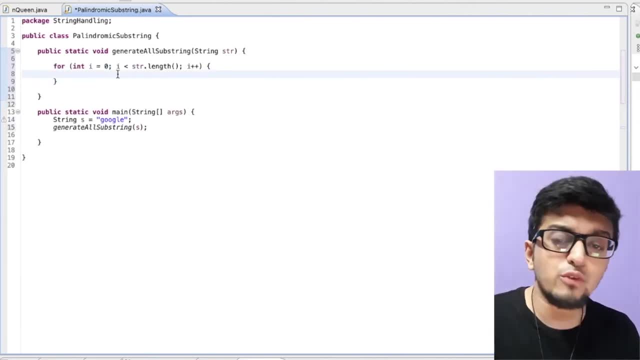 a for loop over here And within this for loop we will be considering each character as the middle of the palindrome. And you know, right now there are two type of palindrom: One is the odd length palindrom and another is the even length palindrom. So we have to handle both the case simultaneously. 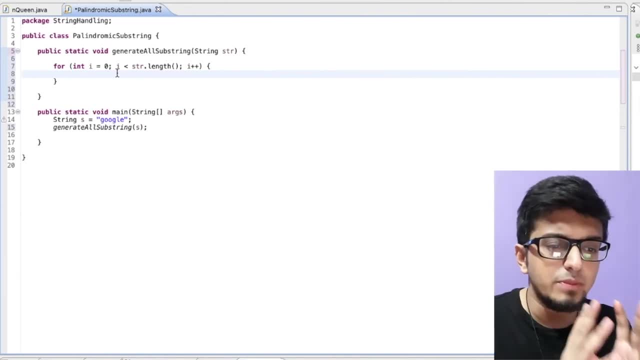 So let's see how we will be doing it over here. But before implementing that logic, I will be declaring a additional data structure called as a hashSet, which will basically store all the substrings that are generated from a string. So let's declare a hashSet over here. 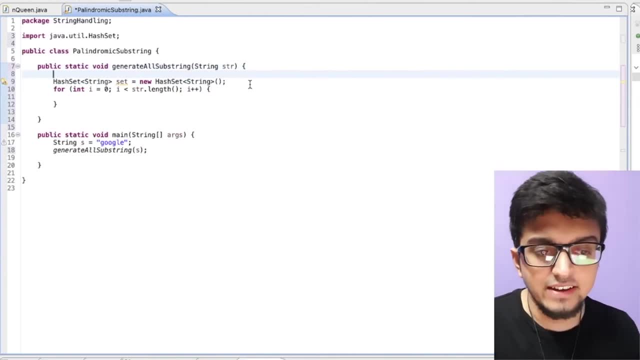 So now we are done with the initial declaration of the hashSet and the following. Now let's write the logic of handling the odd and the even length palindrom, And for that we have to write a utility function which will help us to determine. 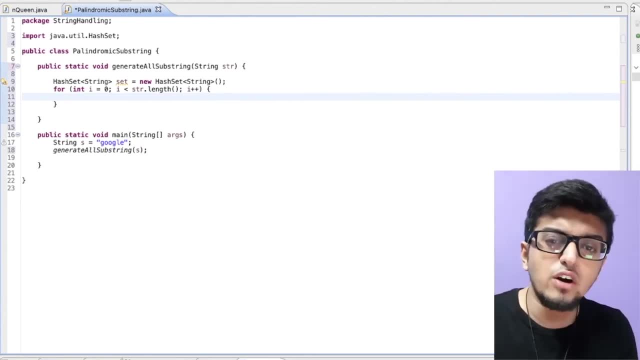 that, whether the adjacent characters which align on the both sides of the middle character are equal or not, And if they are equal, which means that the new string which we are considering should also be a palindrome. So, over here, what we will do, we will call a function called as. 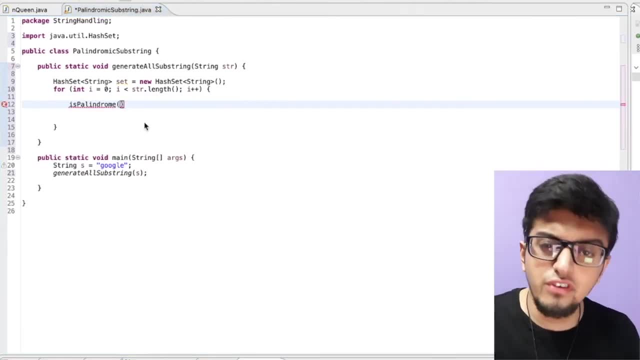 isPalindrome And within this isPalindrome function, we will be passing for argument as our parameter. First is the entire string, Next is the ith index, Next one will also be an ith index- I will tell you why- And the next one will be the set, which is the additional data structure we have declared. 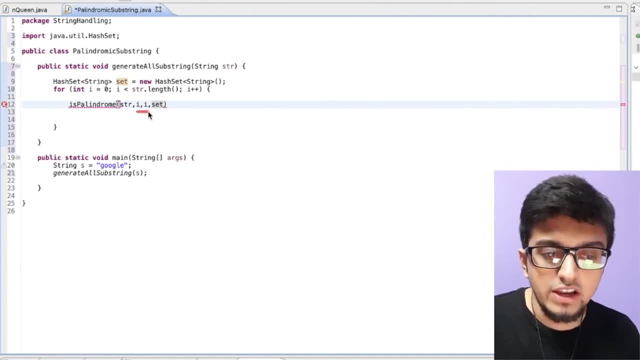 over here Now why I am passing 2i over here. I will be explaining it very soon, But if you have understood already it will be great for you. So just to give you a hint, this function call is responsible for listing down all the palindrom of odd length. So basically this will determine all. 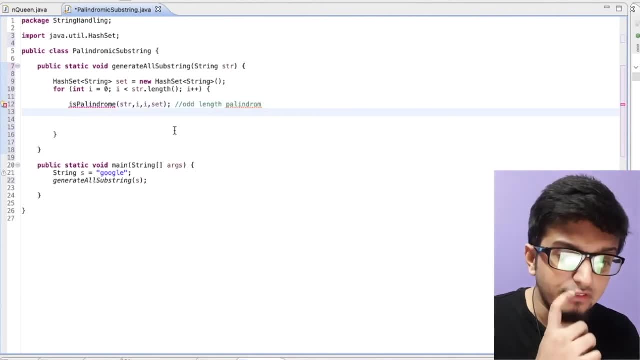 palindroms, And the next function that we will be calling from here is for the even length palindrome. So we'll copy the same functionality over here, and over here, instead of passing i, we will be passing i plus 1.. So I hope this is clear to you why I am passing 2i over here and 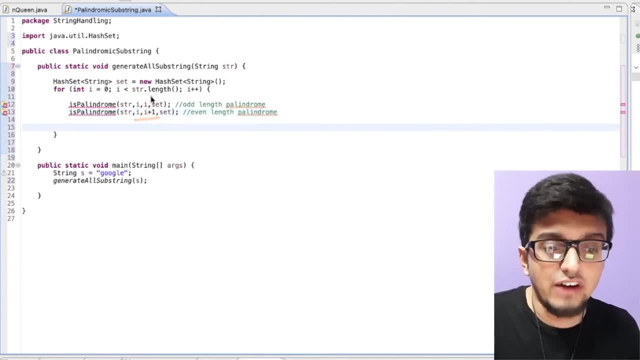 why I am passing i plus 1 over here, Because of the fact these are actually determining the window size of our palindrome. So, as I have already told you that for the odd length palindrome, we are passing the window string at a time And at our initial stage, the value of i or the value of the. 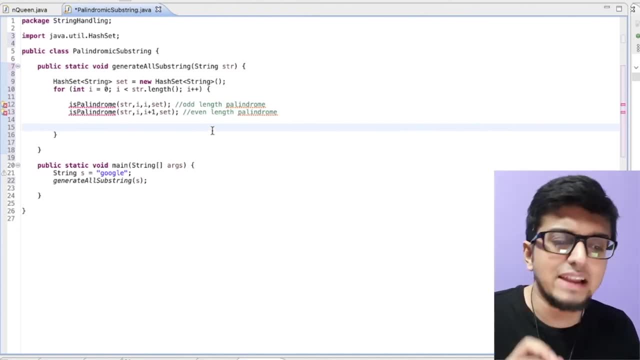 window size is 1.. Whereas in case of the even length palindrome, the value of our window size is 2.. Which means that we are considering two characters at a time, And that is why over here we are sending i and i plus 1 over here. So now, if you guys are clear with this concept, let's 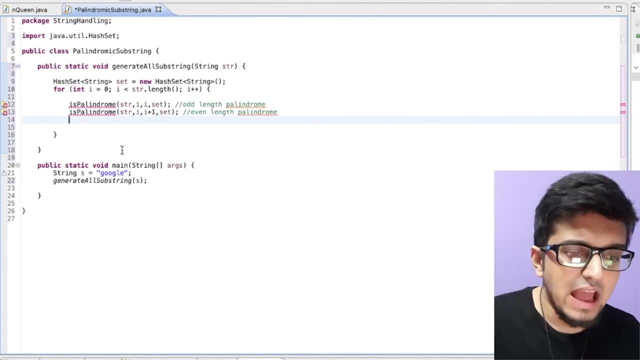 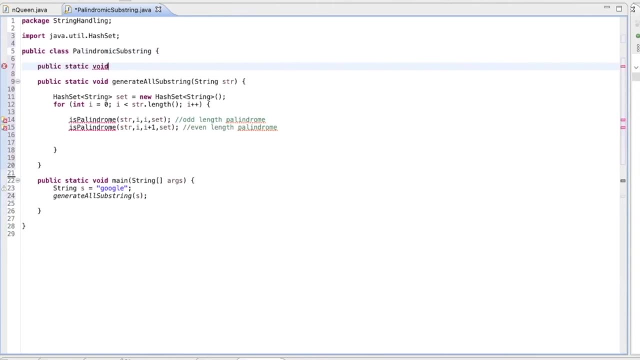 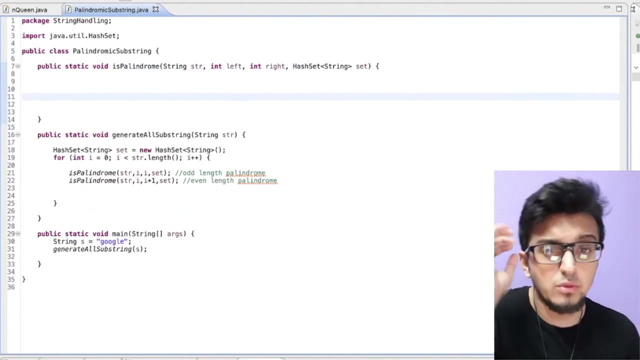 proceed with implementing the function that is isPalindrome, And the logic for isPalindrome is very simple and straightforward. So let's first learn how to use isPalindrome. So let's define the method over here Now. over here, we will write the main concept of finding the palindrome. 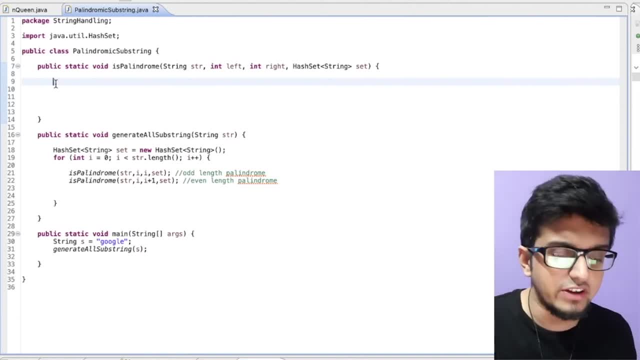 So let's see how we will be validating the palindromic substring over here. So what we will be doing over here. Over here we will be writing a while loop. Now, why over here, I am writing a while loop, you will get to know very soon. But let's first write the while loop over. 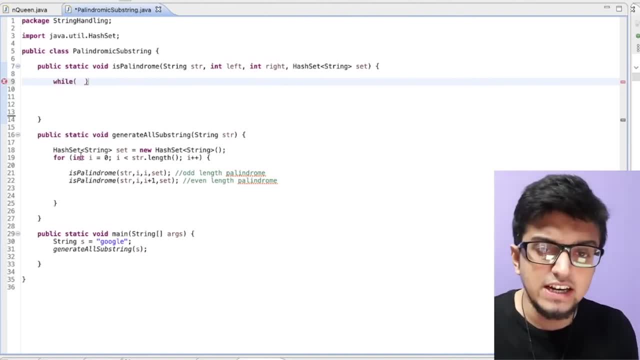 here And within this while loop, we will be putting the condition that, whether the left hand side pointer is equal to the right hand side pointer or not, And if they are equal, which means that the substring that we got till now is a palindrome, And if it is equal, we need to again. 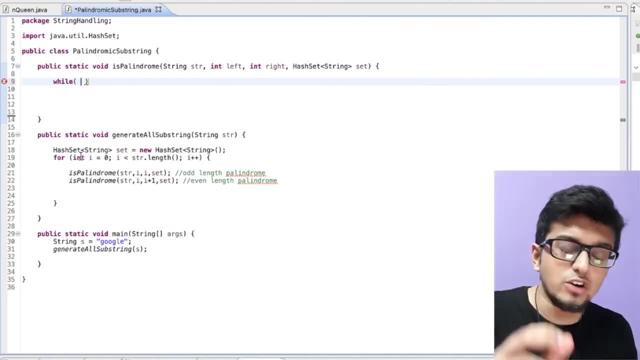 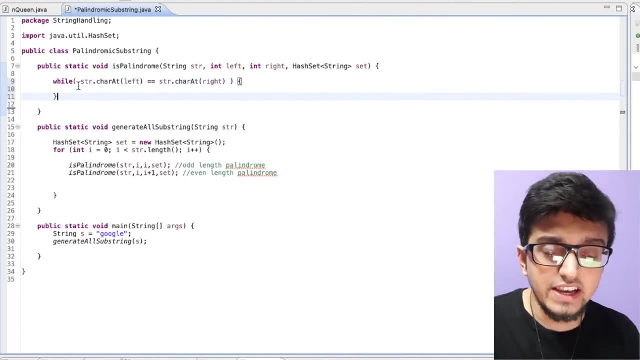 extend our window by size one. So let's implement that logic over here. So what we are doing, we are just checking the left hand side pointer with the right hand side pointer And if it is equal, then what we have to do, we have to increase the size of our window. 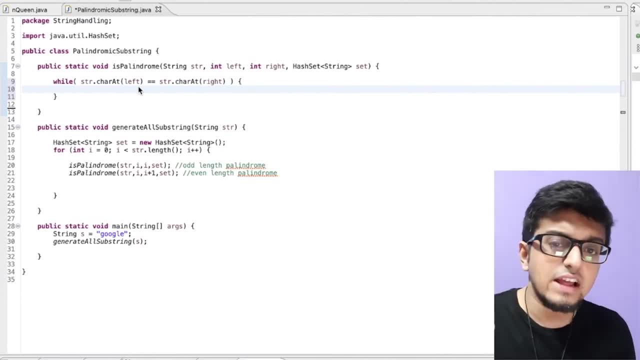 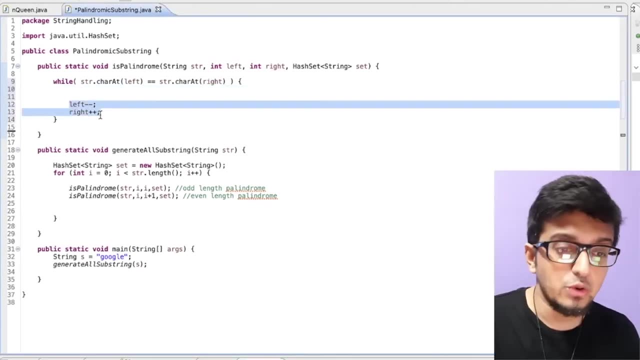 And for that we have to move the left hand side pointer more towards left and right hand side pointer to the right. So I hope this logic is clear to you. So now what we have to do, since we already have validated that this string is a palindrome, which means that all the substring that are entering within this block 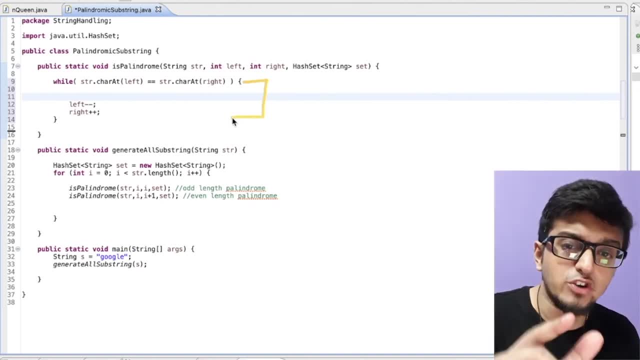 should be a palindrome, And for that we have to store that palindromic substring within our hash set. So we'll store the palindromic substring within this hash set And this is basically the entire logic of our algorithm. But one more condition you have to. 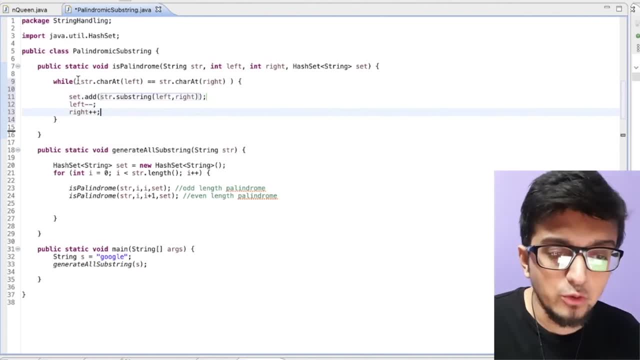 put over here, that is over here. we have to put a termination condition over here. That is, we have to check that our left hand side pointer should be always greater than zero and our right hand side pointer should be always less than the length of the string. Otherwise, you know, we will get an. 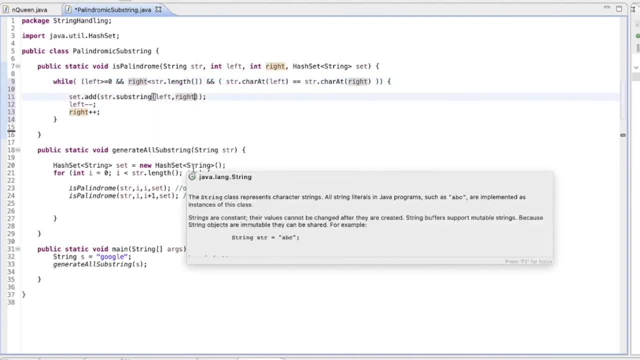 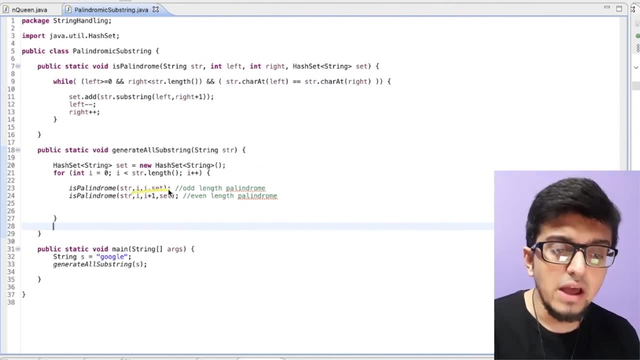 exception over here. So hopefully this logic is clear to you. So what we are going to do is we are doing over here for the first time- we are checking all the odd length palindrome and that is why we are passing a single length character over here And over here in this function we are checking 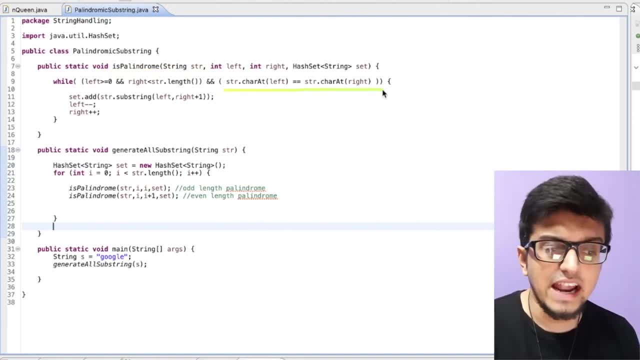 whether it is palindrome or not And obviously, since it is a single character, it should be palindrome And thus it will go inside this loop and it will add that single character within our hash set. And since this is the palindromic substring, we have to increase our 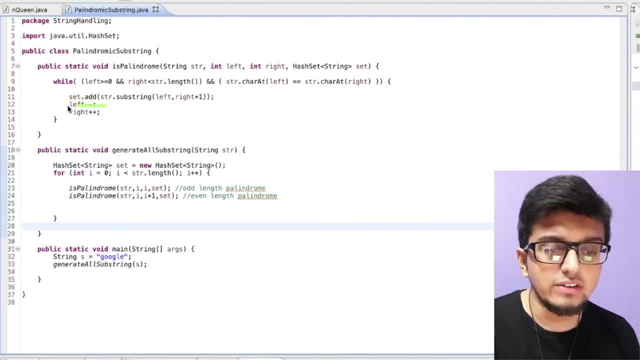 window size, and thus we have to increase our left pointer towards left and we have to move it to the right pointer towards right, And in this way we will be keep on checking each and every substring that, whether they are palindromic or not, And as soon as one of this condition becomes false, 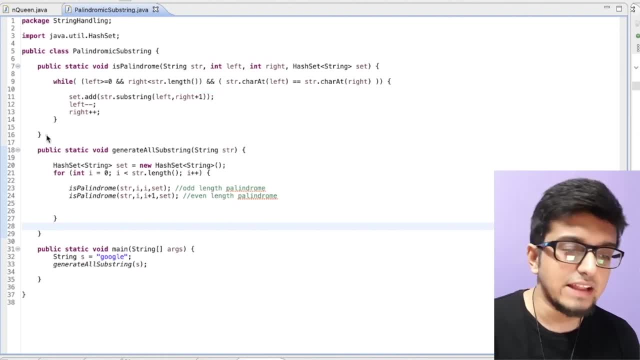 the loop will terminate over here and we will come to our next statement that is over here, which is actually determining the event palindrome over here. So I hope this is clear to you. If not, please do a dry run of this code so that it will be much more. 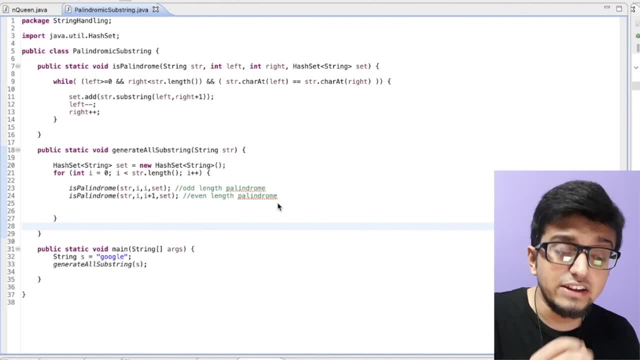 easy for you to understand the code. Now, in the last and the final activity that you need to do over here, and that is we have to print the entire palindromic list over here. So for that, I will be putting a sysout over here And over here I will be printing the entire set which we 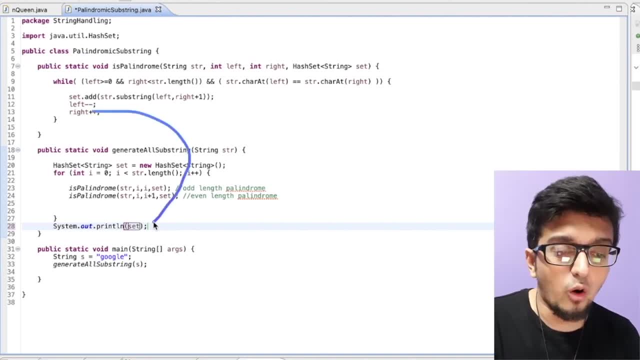 have generated from here, which is basically containing the all the substrings that are possible to generate from a given string. So let's run this program and let's see whether we are getting all the output as expected or not. So let's run this program and great, you can see. 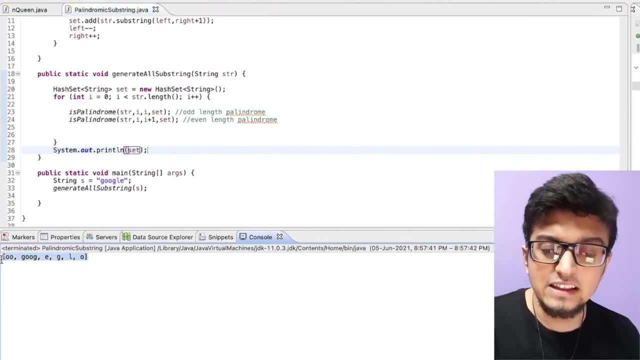 over here. we have got all the palindromic substring that is possible to generate from this given string, which are nothing but all the characters over here. Apart from that, we have two more string, that is, 00 and GGG. So I hope this is quite clear to you right now, that how, with the help of simple, 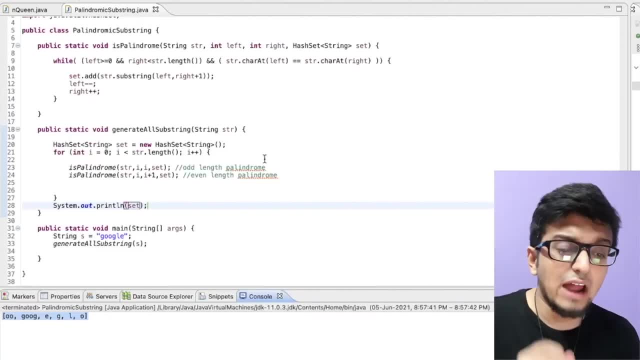 line of code. we have implemented this whole algorithm. And one more enhancement. I want to show you over here that how, with the help of this algorithm, you can find out the longest palindromic substring over here. So for that, what I will be doing, I will be declaring a variable over here. 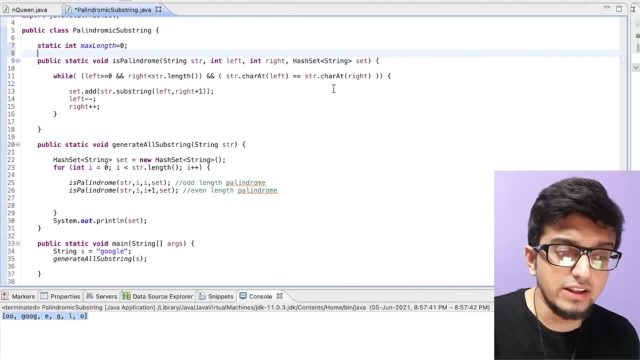 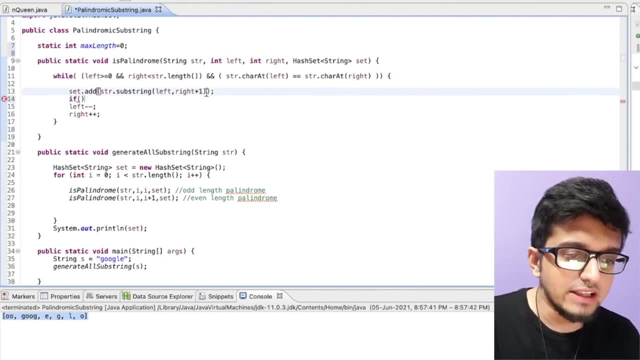 called as maxLength And over here within this function, as soon as I'm getting a substring as a valid palindrome, I will be putting a check that, whether the length of this substring is greater than the max or not, And if the newly generated substring has a length greater than, 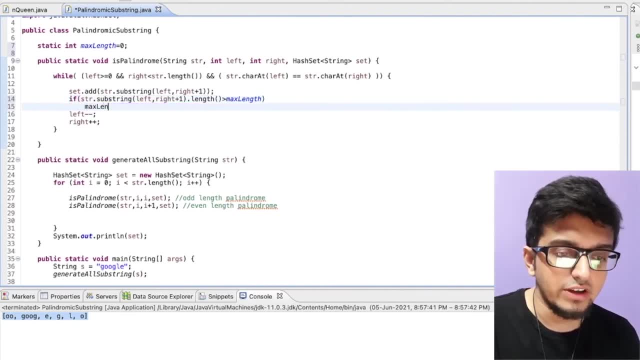 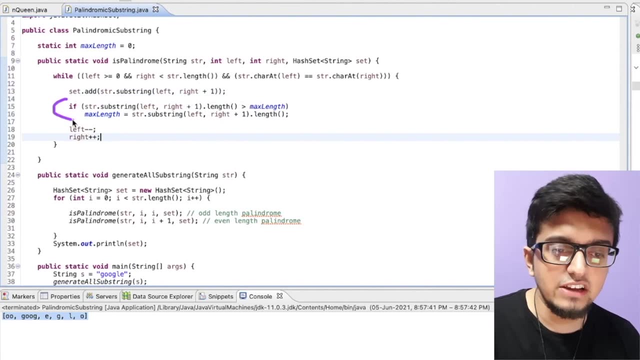 the max length, then we just need to update the max length over here, And that's it. With the help of this simple check, you can easily find out the longest palindromic substring that exists within your string. So let's also print out over here.